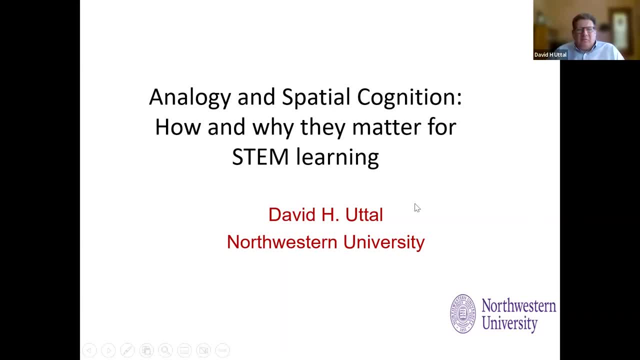 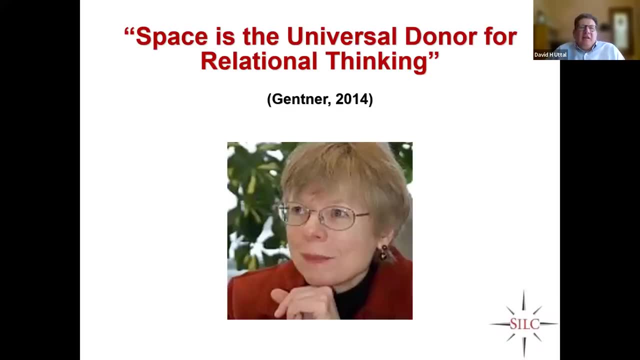 And I'll begin with a quote from one of the leading researchers in analogy and my esteemed colleague, and that's Dedry Gettner, and she said that space is the universal donor for relational thinking. And that was said in 2014 in Riga, Latvia, And I remember it well because I said, wow, that's really, really, really insightful. That could make a big difference. 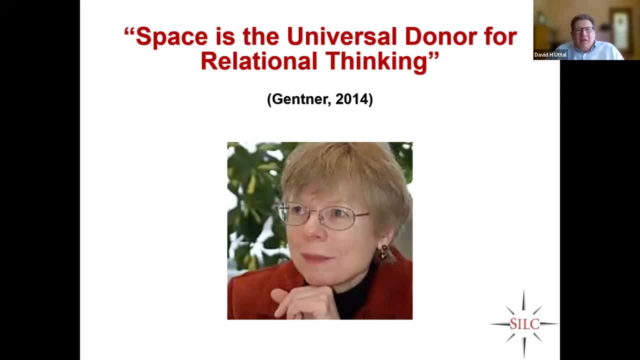 And I've been for the last eight years or so reflecting upon this, And I think that's one comment, because I think it really captures a great deal about the relation between space and learning in science, technology, engineering and mathematics- what we in the United States call the STEM fields. 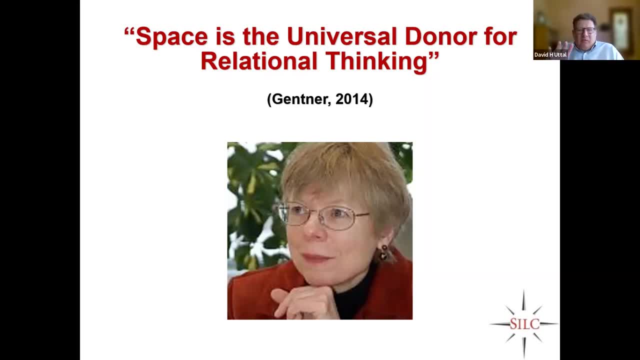 So I want to start with this quote and then I want to- I'll be returning to it at different times- to think about how and why it might be true and why taking this perspective, which is a relational, focused perspective on the relation between space and learning. 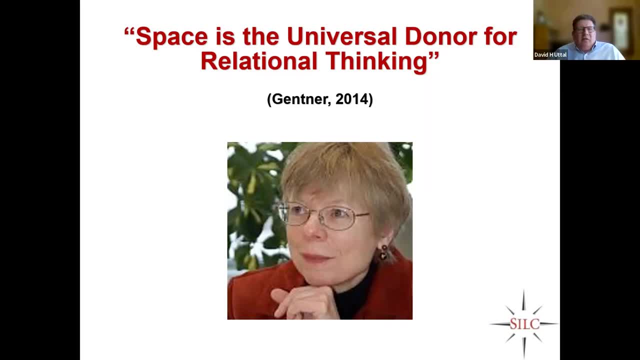 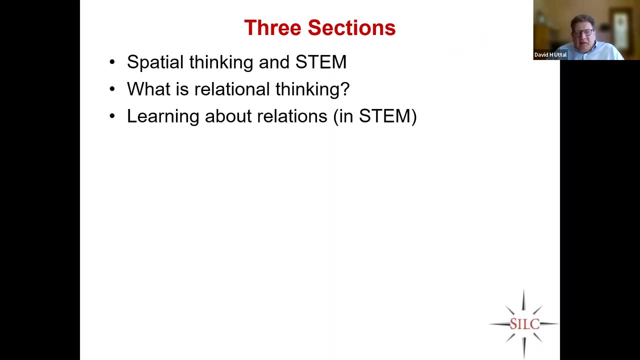 between spatial thinking and STEM learning. Okay, So I'll start off with information to show that spatial thinking is related to STEM learning, which now I think is very well established. There's been many studies that have come out in the past five years or so that strongly show this point. 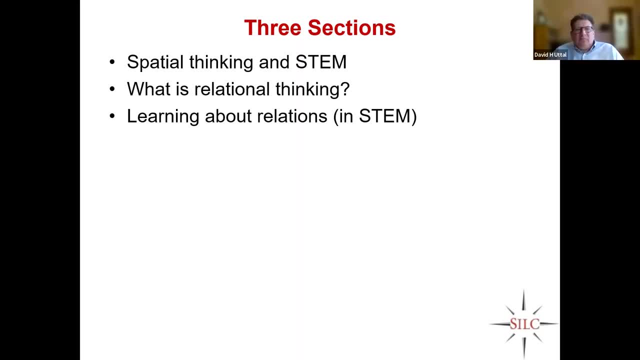 I'll talk about what I mean by relational thinking, or what the field means. Then I'll talk about learning about relations in STEM And how that relates to spatial thinking. Okay, So let's start with some well-known anecdotes from the history of science. 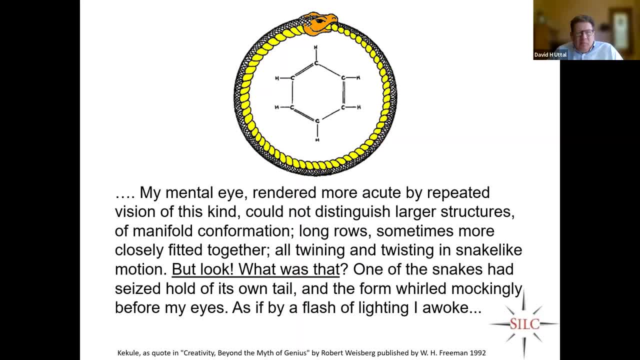 Kekulé originally. most of these tales may well be apocryphal, but they also make the point very well. So, Kekulé, the most important discovery in the history of organic chemistry, arguably when he discovered the structure of the benzene ring. 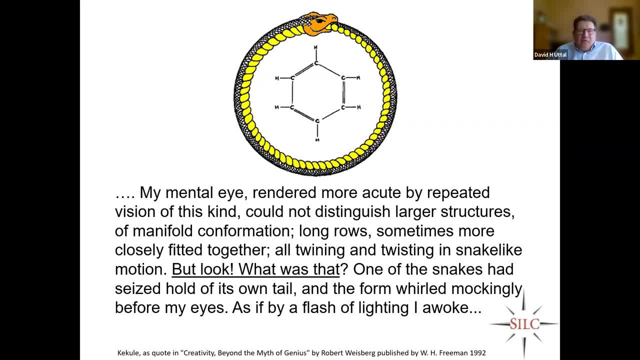 And first of all, it demonstrates The importance of spatial structure, because he knew what the elements were, but he didn't know how they were arranged, and how they arranged is incredibly important in understanding their chemical properties. Now he supposedly dreamt of a snake biting its tail and I never fully understood until about a year ago how you get from that to the hexagonal structure. but it was simply the ring idea. 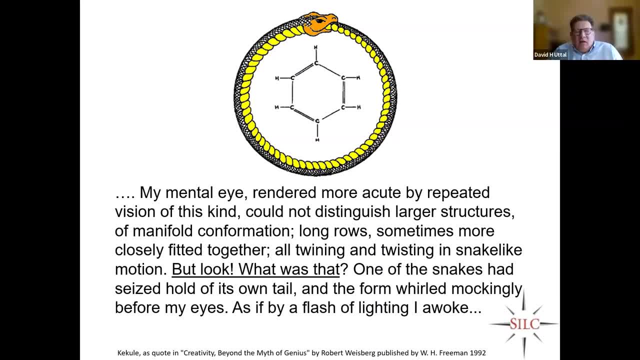 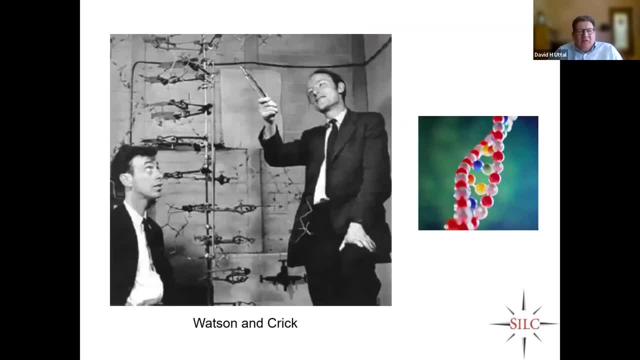 The, the- the hexagon followed from The idea of a connected figure, And so this is one example um. a somewhat more recent example is the history of the um discovery of the DNA molecule. Watson and Crick working on the um, the, the, based on the work of Rosemary Franklin, um, discovered this double helix idea and lots of different groups were working on this. 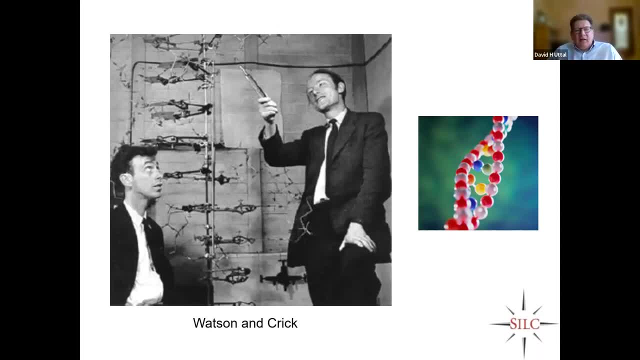 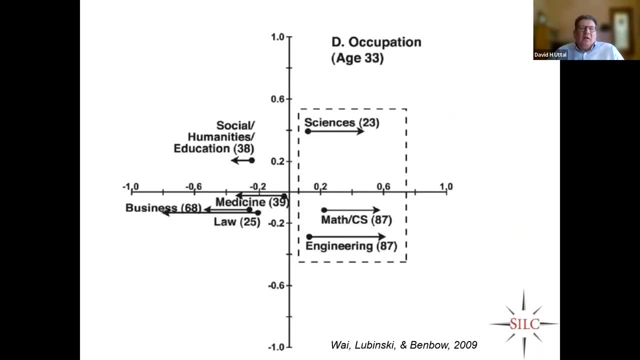 They all had the uh components, but it was the critical insight, Yeah, Into the spatial structure that allowed them to have this great insight about explanation. Okay, So these anecdotes are are useful, but, uh, there's a lot more empirical research that strongly suggests that spatial ability is related to STEM achievement, attainment, persistence, any of the measures, and even creativity, any of the measures that we care about in in trying to understand who succeeds at STEM, who continues to succeed at STEM and who continues to succeed at STEM. 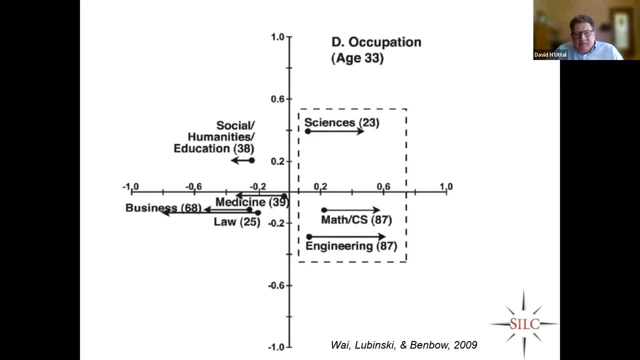 Well, you know I'm. you know I'm so sorry to hear what I'm not doing. of course I'm sorry. Well, I'm so sorry to hear. are you surprised that there's a gap at the top? That was, that was almost there. 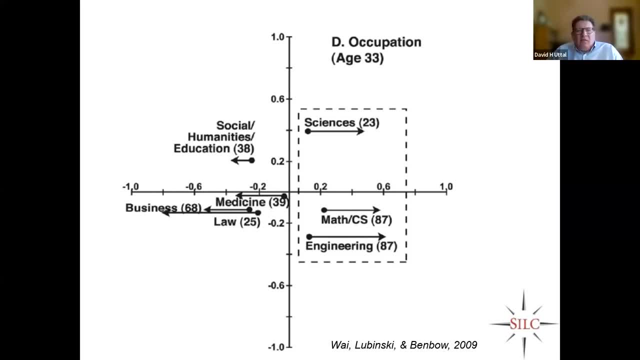 I'm just joking, It's okay. Of course there's a gap right there. There are egg дом. Hari, I'm cks from FTAP, like I don't want to say it too exactly, But I'm just began as a innovative consumer Legion, or it's not that I'm, that I'mievoe know. 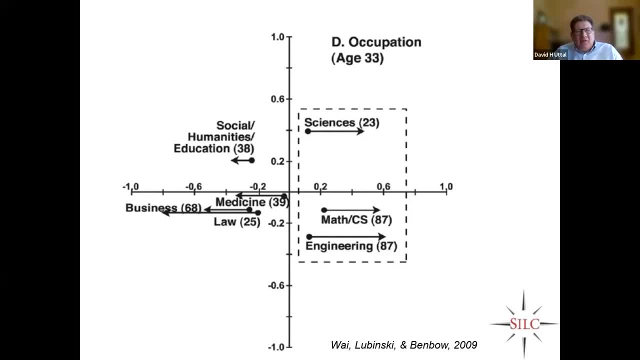 Well, You went into Hajj with the X, right? Yeah, Yeah, Okay. So let me answer that. Okay, extra value obtained by looking at a spatial ability score in predicting who went into STEM fields. So the X and Y are normalized, I believe SAT scores, And so a score of zero. 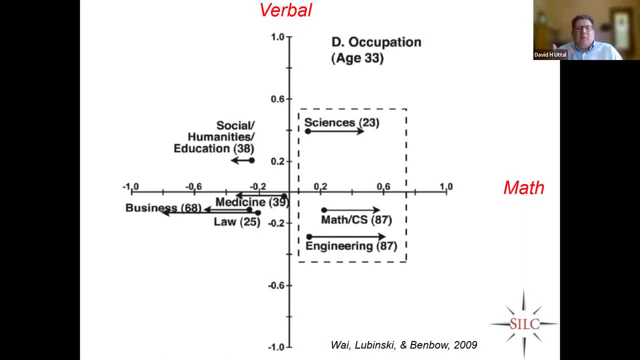 is average. So just looking at X and Y you could see like people who went into sciences had the other they're actually they're good at everything They're. they're relatively strong at math, at verbal and at spatial. This arrow represents how much extra predictive. 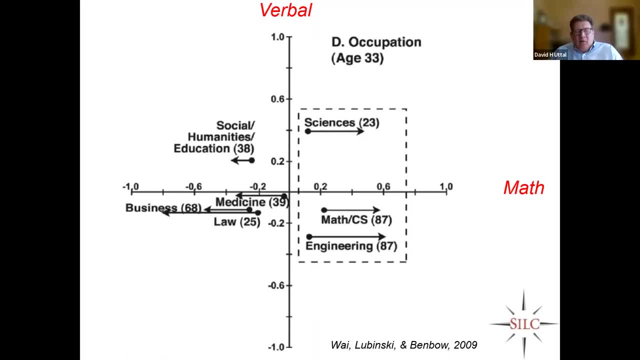 power you get from knowing the spatial ability score above and beyond the verbal and math, And it's quite a bit. in some of the STEM fields it's actually more than math or verbal. Now, these negative predictions are not. they're not saying that people are bad, It's just. 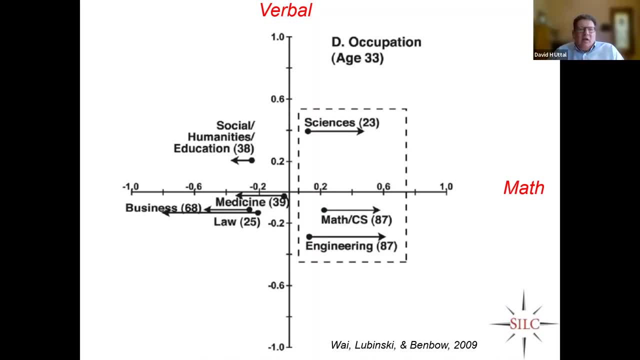 relative weighting or tilt of abilities. So these negative predictions are not. they're not saying that people are bad, It's just relative weighting or tilt of abilities. So these negative predictions are not. they're not saying that people are bad, It's just relative weighting or tilt of abilities. So 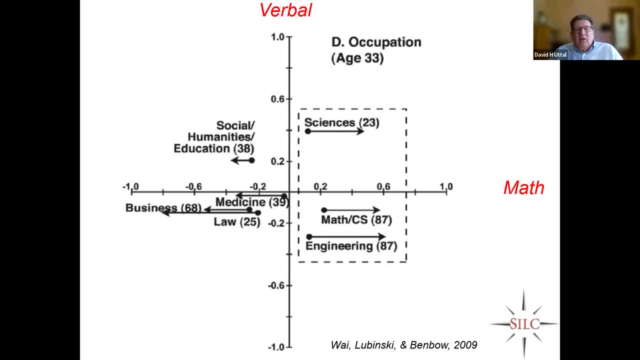 these fields, and this is quite old data. It's the only data set we have that's nationally representative and that included spatial ability. It desperately needs to be done again so that we don't have to keep citing work that started in 1960, but it's. it's what we got, So I'm 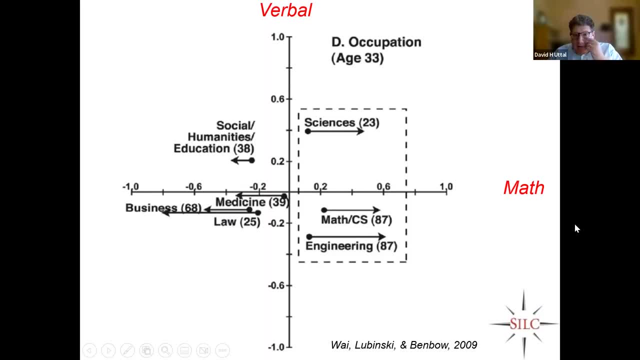 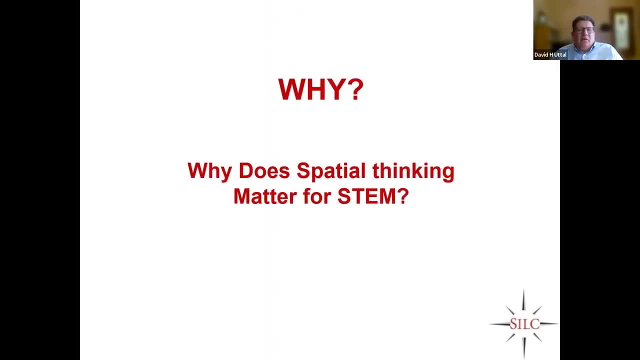 sure, some of these have changed and there's some cohort effects here, but still it strongly shows there's a relation between spatial ability and STEM outcomes. Now the question I've been addressing for some time is why? why does spatial thinking matter for STEM? 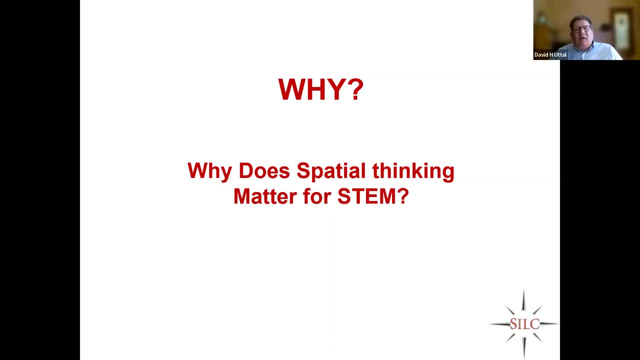 And there are lots of overlapping reasons and none are necessarily mutually exclusive. but I want to try today a general integrating hypothesis that the fundamental reason is because science is about relational science and mathematics, or at least some of the critical learning challenges, are about relational thinking. 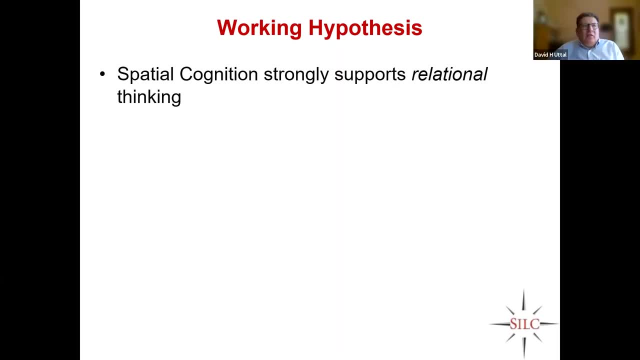 And, as Dedry suggested, spatial cognition and spatial representations strongly support this relational thinking. So relational thinking is a key characteristic of human thought When we, like Gettner and others, have shown in the history of science that there are very important discoveries that were based on the process of analogy, And you can predict both where people 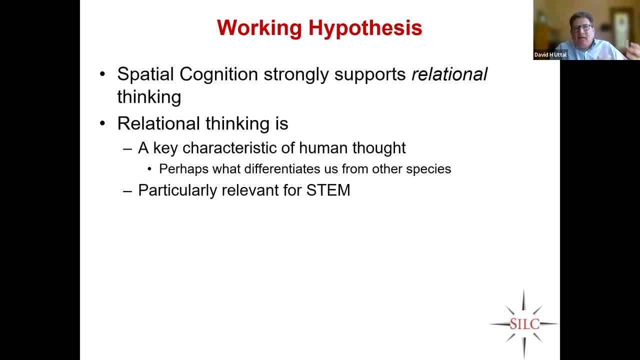 went right And some of the uh certain paths and wrong turns that they took. and relational thinking is particularly relevant for STEM. I would say that to some extent, STEM learning is learning to think about different kinds of patterns and relations, So STEM is all about relations. Students do well when they think about STEM topics relationally. 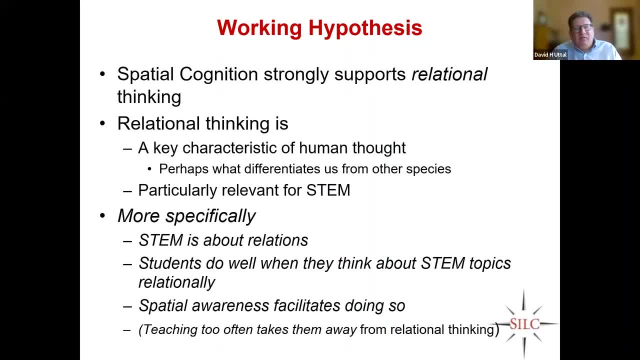 So a lot of expertise, and classic examples are, in physics, for example, are that the experts can reduce, you know, one of these enormous textbooks down to a few categories based in part on how they relate to fundamental forces in the world. So they can take Newton's three laws. 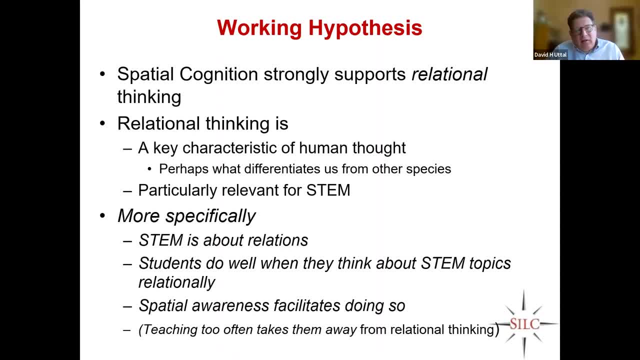 and relate every problem to it, And, in contrast, the novices are sort of stuck in surface properties like this is one about inclined planes or this one is about pendulums- And they often can get it right, but they fail to benefit in studying a new topic sometimes- or we call it transfer. 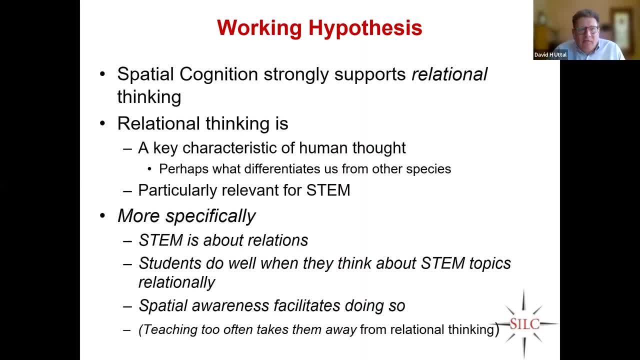 because they don't see the connection, And those connections are often about relational thinking. Good teachers promote relational thinking when they are talking about STEM And I want to make this argument is going to go from about age three or four through college And yes, it's overly bold, but I think there are some connections that when you see the children, 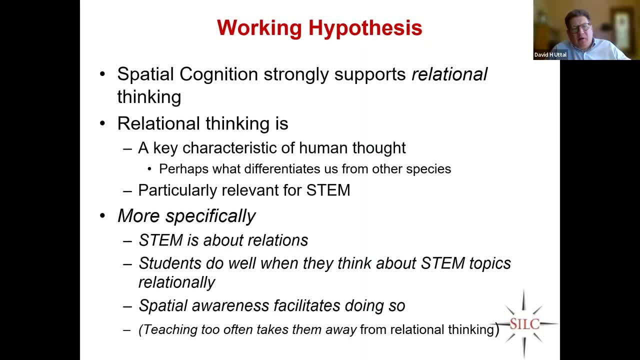 are learning about, for example, the properties of numbers, both symbolic and non-symbolic. part of the challenge is understanding the relational properties of numbers. This, for example, is why we know from Susan Carey, Karen Nguyen, Kelly Mix, many, many others that simply 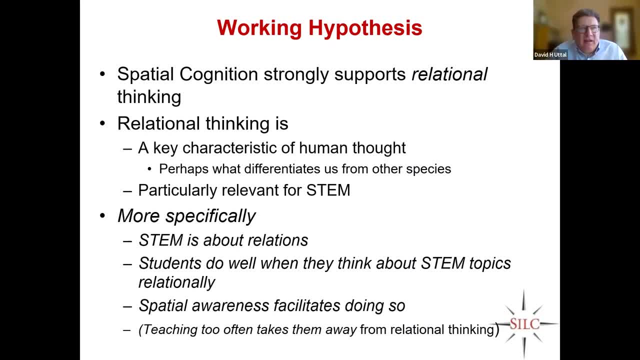 on knowing the numbers is not enough to being able to count in no way proves you understand the integer properties of the numbers you're naming, And part of that is you have to have a relational understanding, And part of that may stem in part from spatial representations that I'll talk about. 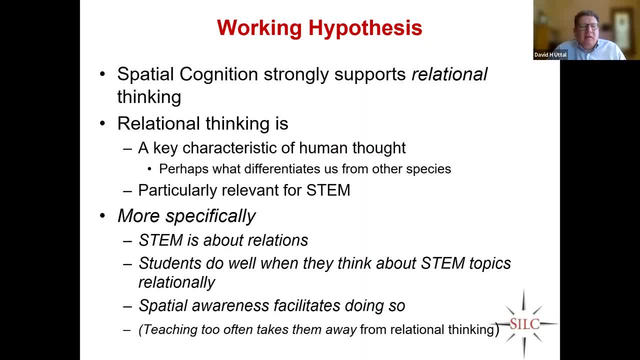 An unfortunate corollary. the last line of this slide is that teaching too often takes them away from relational thinking. Towards the end, I'll give you some examples of how we teach things like fraction and graphs that, unfortunately, at times emphasize precisely the things that relational theory would. 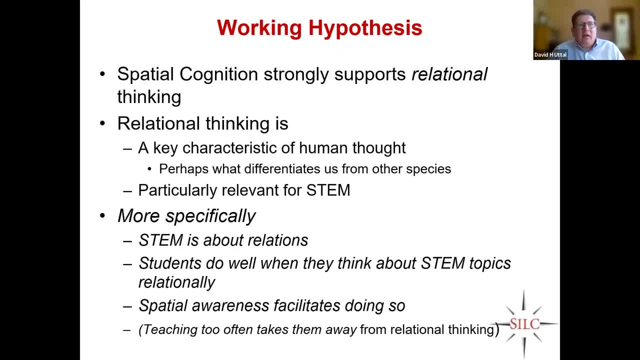 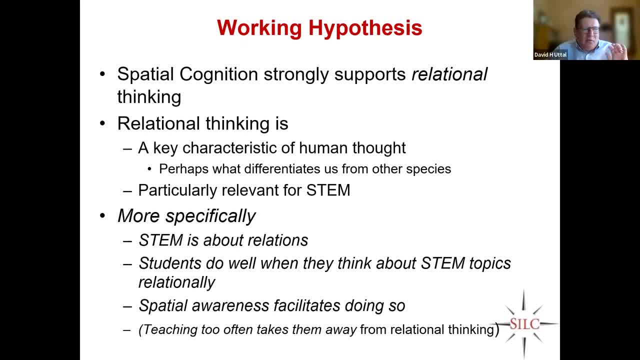 understand that And I think it's important to understand this and this, And I think I'm going to add some exceptions to this- And IES and other agencies have funded lots of great research on specifically this issue. So the situation it's not all bad And we are benefiting from the 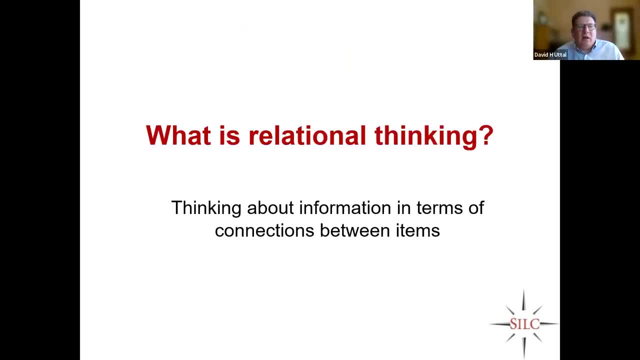 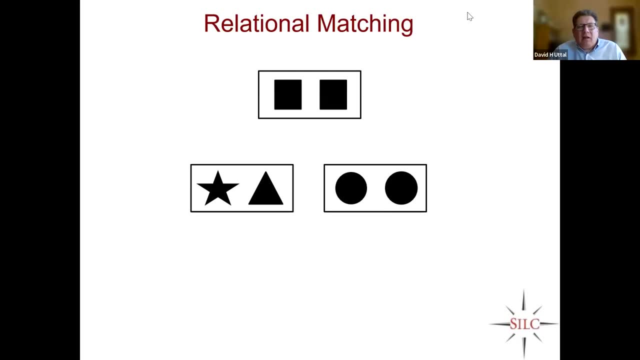 cognitive science of relational thinking in education. So what do I mean by relational thinking? Okay, So this is very well illustrated by example. I mean I can give a definition, But I think these examples reallywhat I do there. Everything okay on your end. 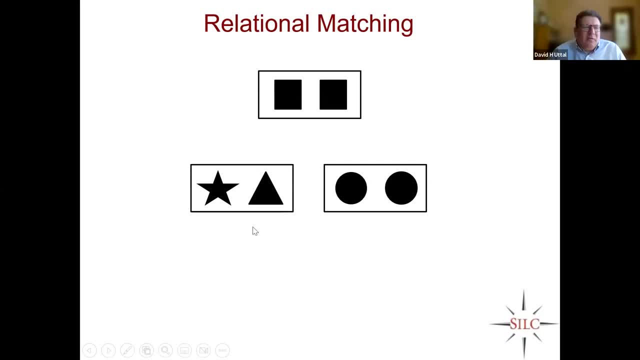 Yeah, Hello, Hello world. Yes, everything looks okay. Okay, thank you, because we're giving you a thumbs up in the, but you probably can't see them. I can't see that. yes, Everything's good so far. No, we haven't seen any change on the slides. 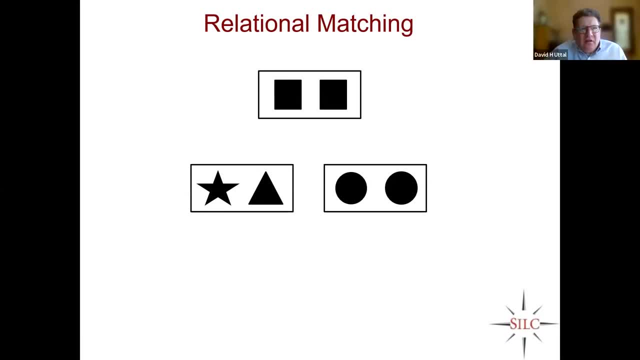 As many people have pointed out- Penn, Holyoke and Povinelli and many, many others, going back decades- the relational match-to-sample task is one that seems to be okay. there's a debate, but can we teach non-human species to do this? 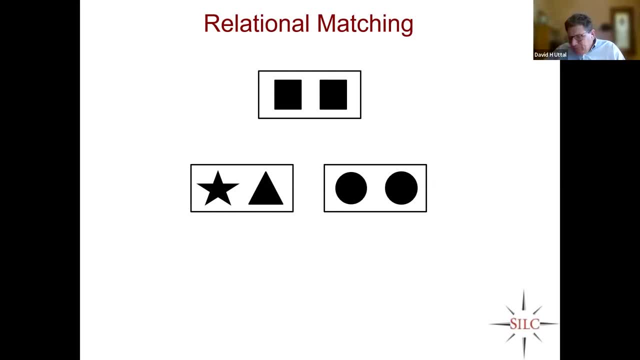 The answer is a definitive maybe, and it's really really difficult. I mean, you have to have a dedicated student who will spend hours and hours and hours reinforcing them and then, after 10,000 trials, you think you got it, and then you switch the stimuli a little bit. 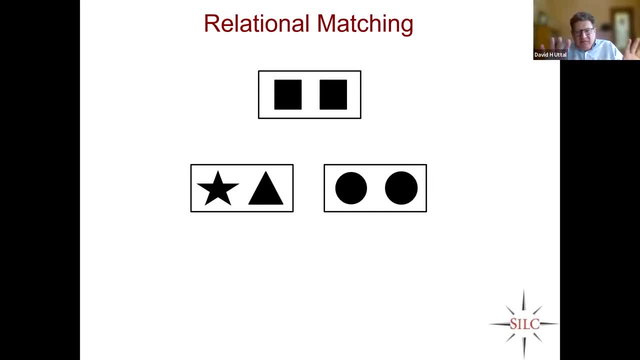 and they go back to zero. Okay, And if you disagree with me as that characterization of literature, that's great. but one thing I don't think you would disagree with is that you know, everybody knows- how smart crows are right. 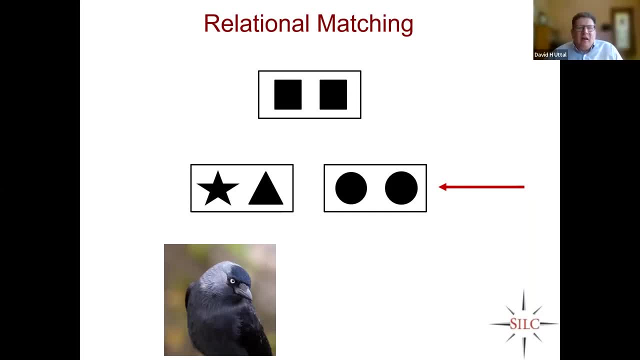 They're scary smart, but they seem to have some trouble with tasks like this, and likewise our close ancestor, chimpanzees. But in contrast, a four- or five-year-old child has no problem doing this at all, and whether it's a difference of kind or not. 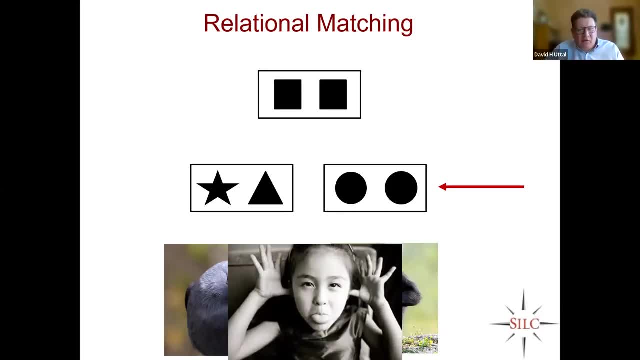 A quantity is an interesting question, but the difference is so dramatic that something is going on, And so these tasks require relational thinking. You have to go beyond the properties of the objects themselves. This is not a question about squares, circles or triangles or stars. 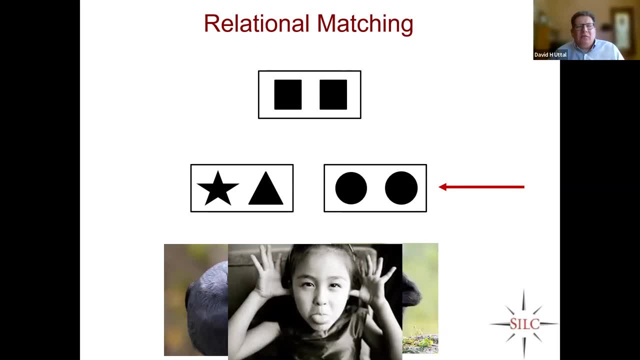 This is a question about patterns and relations, And once you see that the critical pattern here is two-ness, it becomes very easy and you're basically well, You're almost immune to change. I mean, yes, surface changes can make a difference for young children. 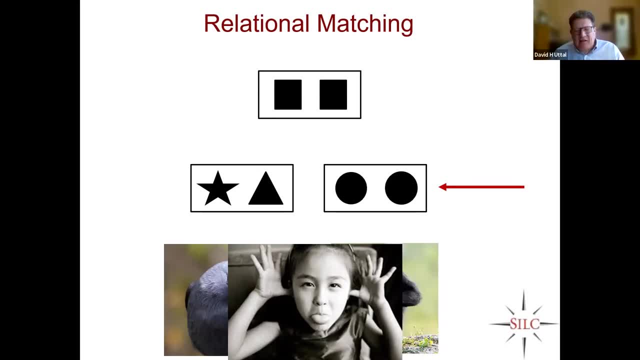 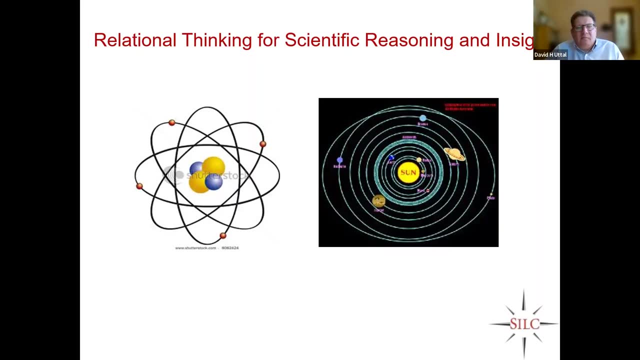 but you know it's pretty protective once you get an insight about the relation, And so we've used this very much in the history of science. Perhaps the best discovery, the best-known discovery is the relationship is using the solar system as a model for the atom. 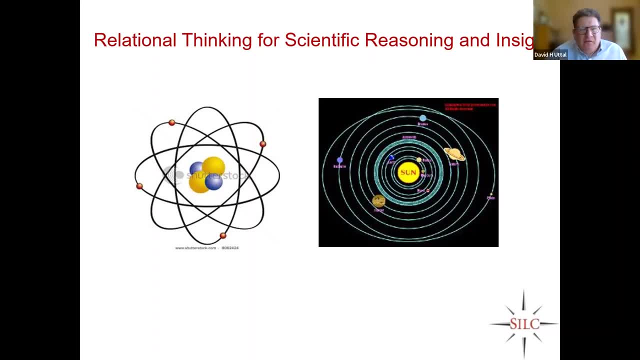 This, of course, was based on 400 years or so of understanding of going from a heliocentric- I mean going from an Earth-centric- to a heliocentric model of the solar system, And the critical thing that's relational here is about orbits. 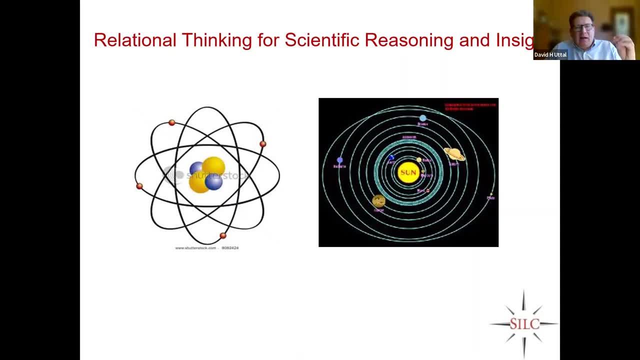 We are interested in how each planet orbits around the sun, and so it maintains that relationship. And yes, each orbit's a little bit different, but that's sort of a secondary fact to understanding the. You can only make sense of those differences. 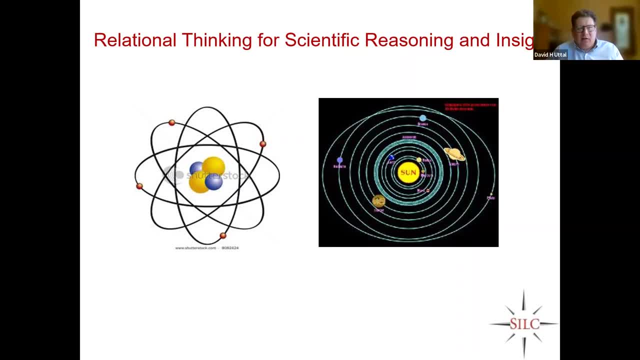 if you understand the general idea of orbit in the first place, And then Maxwell and others mapped that on to the atom structure And although it's far from perfect- it doesn't correctly represent electrons, it does represent a pattern of relations, which is a critical insight for thinking about both the solar system. 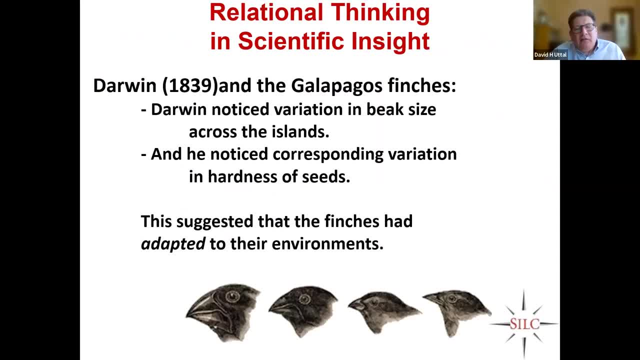 and the properties of the atom. In biology, you know Darwin and the Galapagos finches, I mean. to some extent, the discovery of natural selection depended upon these relational insights. So yes, he went and he observed the beaks. 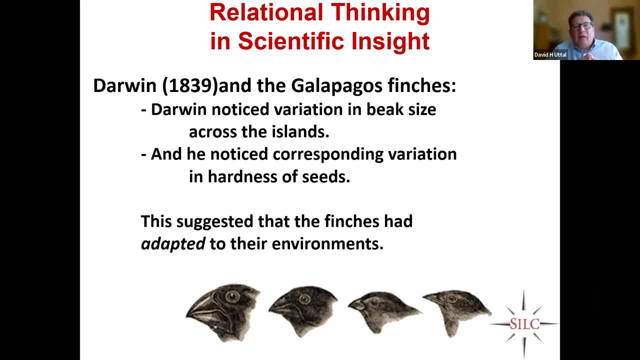 and he carefully measured and things like that. but it was lining them up like this and looking at the similarities and differences that helped him gain an insight. So he could have studied each in isolation, but the comparison and the relational structures highlighted both the similarities and differences. 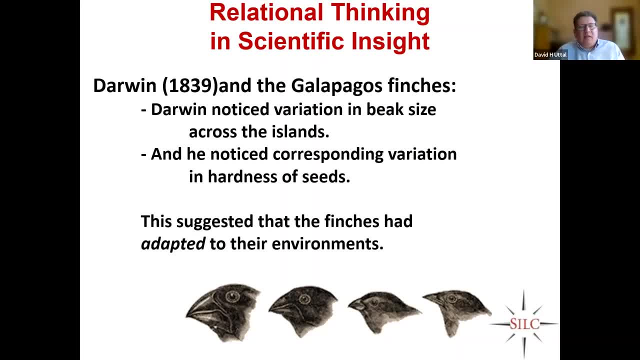 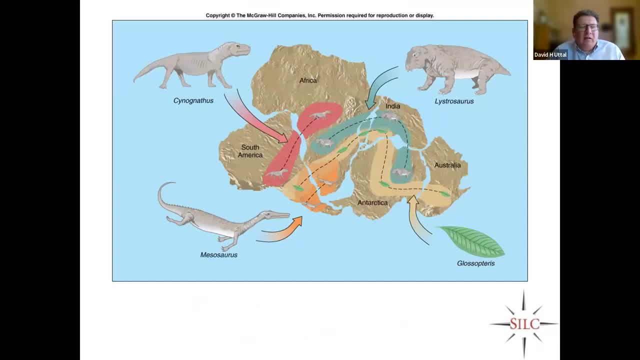 And that was a contribution to the insights that found the foundation of evolutionary understanding. This is one of the most important representations in the history of earth science. It was critically important to understanding the continental drift or plate tectonics, And they didn't have the tools like now we can directly measure movement of continents. 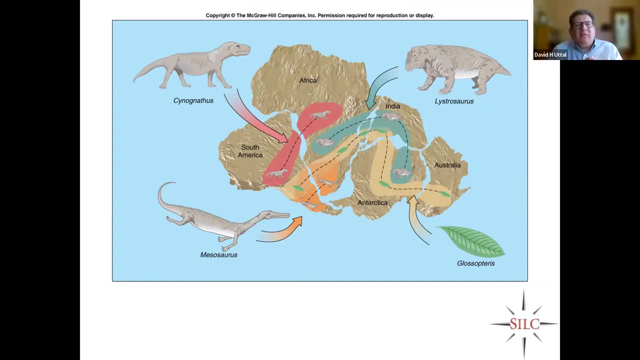 a hundred years ago, Those tools were just in their very conceptual infancy. So this is a process of scientific deduction. It's a pattern of the fossils in relation to speculations about the shapes of continents and how they might fit together. It's very hard to explain the pattern of fossil distribution. 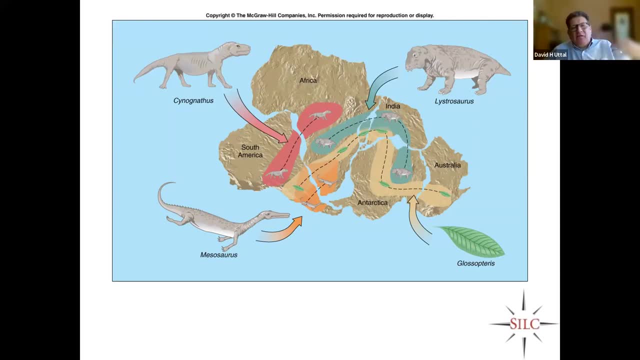 without taking into account the geology. So it's the paleontology combined with the geology and those two sets of patterns together and, i will argue, the visual representation of those that made this insight possible. so the general point i'm trying to make is very important. 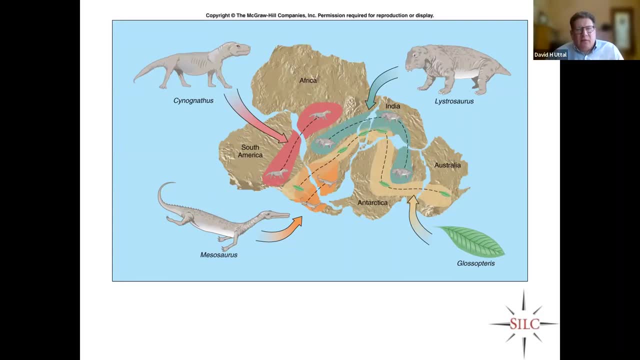 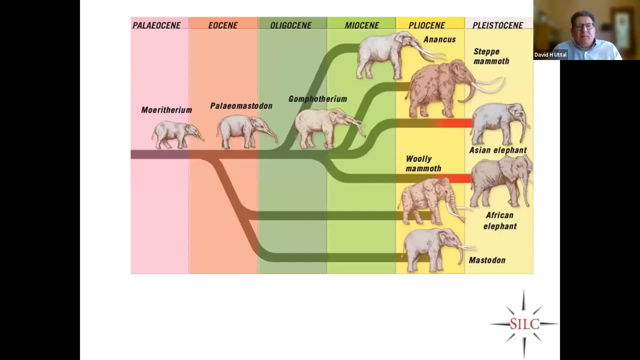 scientific discoveries are often both relational and spatial, and i think there's a reason for that. okay, and then. so we can also use spatial representations to think relationally about non-spatial information. we're so used to seeing these cladograms when we think about evolutionary relations that it's hard to imagine this without it. but there's no um inherent spatial relation. 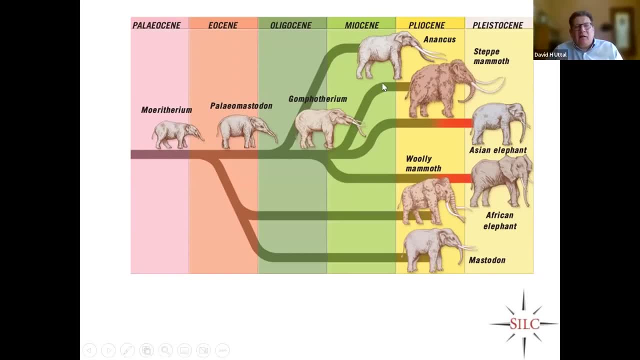 between these games, once we put them in this, in this uh diagram, which is, you know, literally millions of years of time about the evolution of elephants, uh, and how they were related and what split off from what you know and it can be deduced from from dna and from the fossil record. 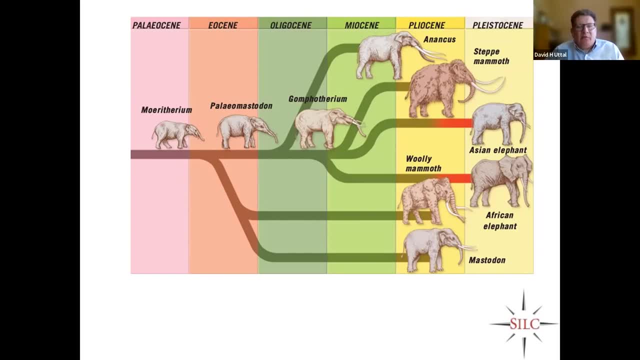 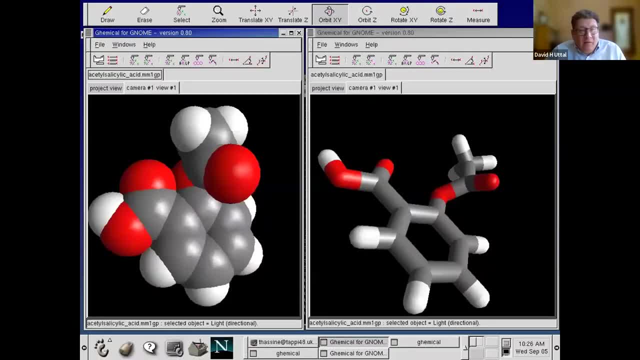 it's called, not because i'm policy wrong, but if they were to right it would just praise visual representations. but here's a good example: where it would helps is equal in condition to the and in chemistry likewise, okay. so this is the kind of thing that we ask organic chemistry students. 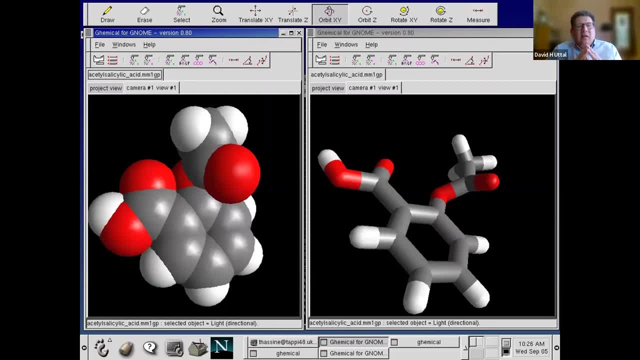 yeah, to do is to see similarities across different models and different chemistry teachers, uh, have different, um uh, favorite models. some of mode models. then put it out in the sun to help that, yeah, but someone like that wants to do it better than i am in the Sacramento过. 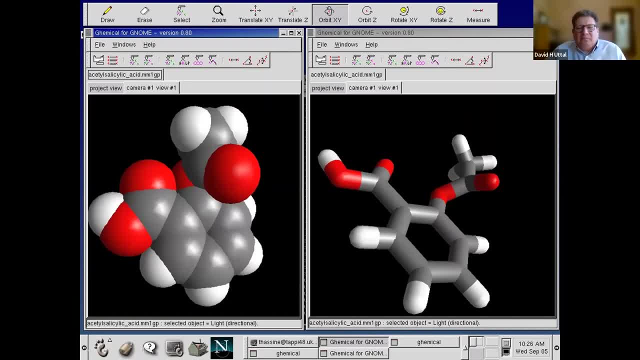 So I think the best thing is simply to continue going, because he will eventually calm down. So if you think about how are these two things related? Well, the first thing that pops out to you is their colors are similar, and that's kind of the concrete, object-based understanding. 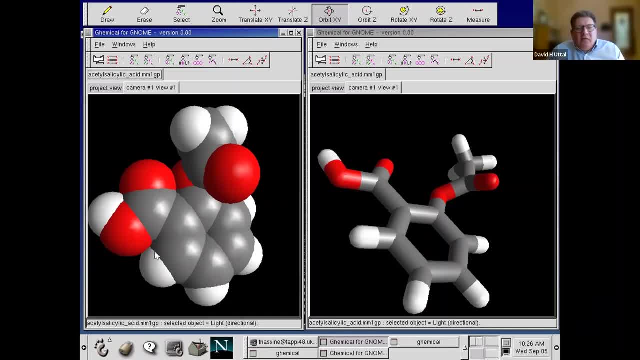 that can give you something of a foothold. But then you start looking for common structure. something about this ring looks similar here and you start realizing that this is a more abstract representation than this is. In some situations it helps to have the details. 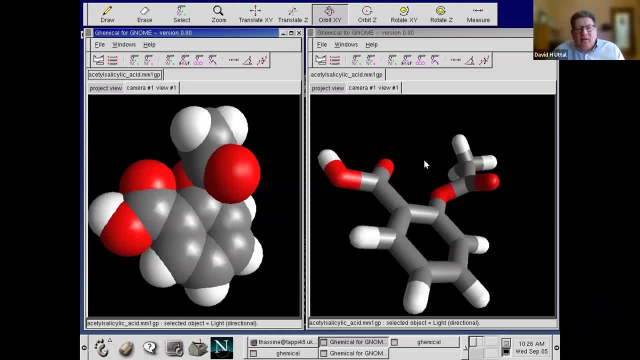 and in some it doesn't. Our ability to think relationally allows us to make insights about common structures and to start to learn the foundations of organic chemistry, And it's interesting in the history of chemistry that we thought a great deal about relations. One: 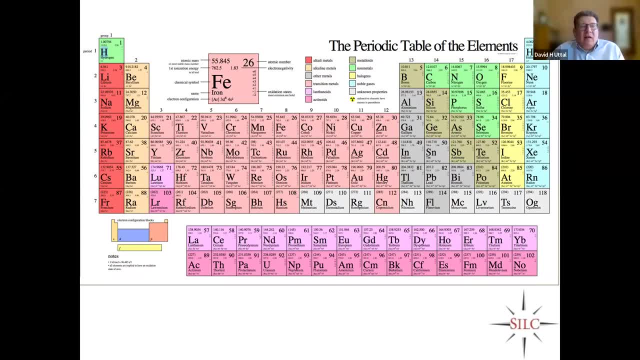 of the beautiful things about this representation is it organizes, what is it? 118, I don't know- a lot of elements in a very specific, theoretically motivated or coherent way And, as any good scientific theory does, it allows us to make predictions. So it's pointed out atoms that should exist. 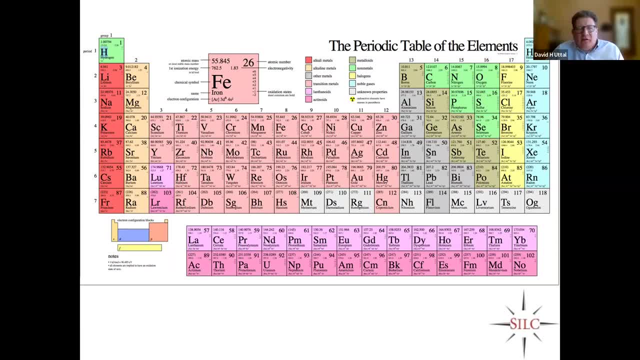 but don't in nature, because the conditions aren't right. but then people have been able to make them in accelerators or things like that, And they knew precisely what to look for. So this is very, very relational and structural And this is, I think, a history. 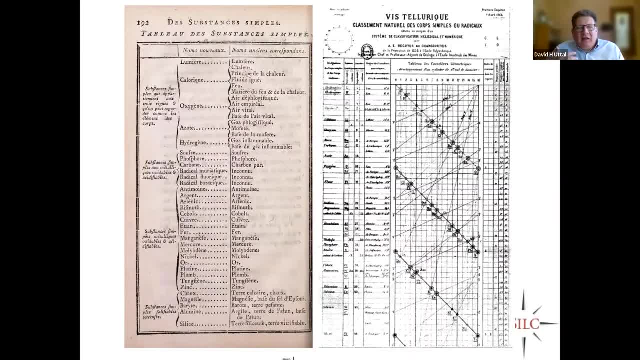 of sort of trying to understand relations between elements, And it doesn't look like our periodic table, but you can definitely see them struggling and using the representation to try to figure out some of the relations between them. So when we have a complex set of data like this, we can clearly see: hey, there's this thing here, This thing's not. 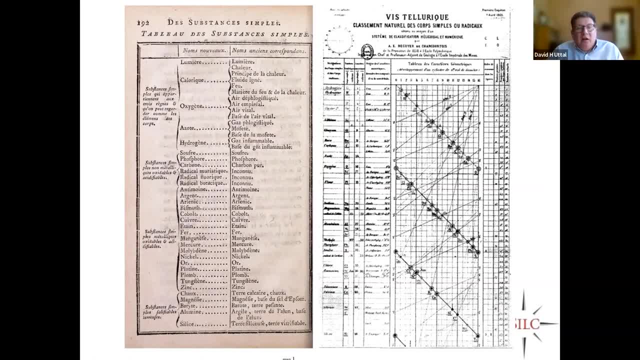 this. we're almost- it's almost- impossible not to start drawing it out- trying to think about relations and, as i'll show you in a few minutes, students whose drawings are more relational, uh, do in fact do better. so this is about taking advantage of the universal donation. 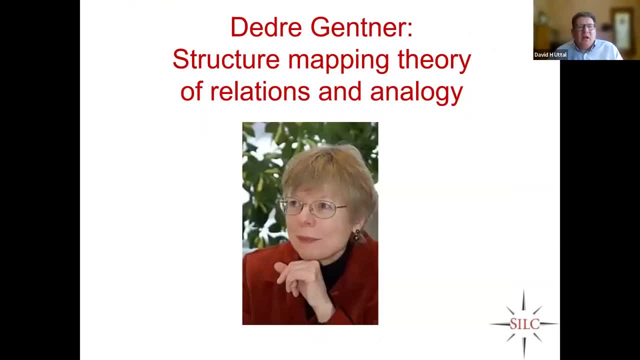 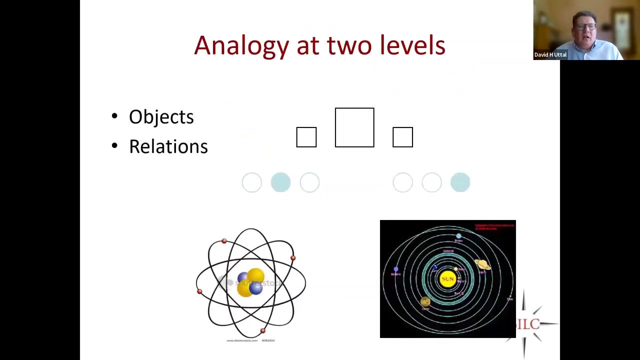 that the spatial representation can provide. so, as you've already heard, i'm relying in part on theories by gentner and markman and others about um, how relations and analogy are alike. relational thinking is the foundation of analogy, um and spatial representations promote that. so analogy can be thought of at two levels. 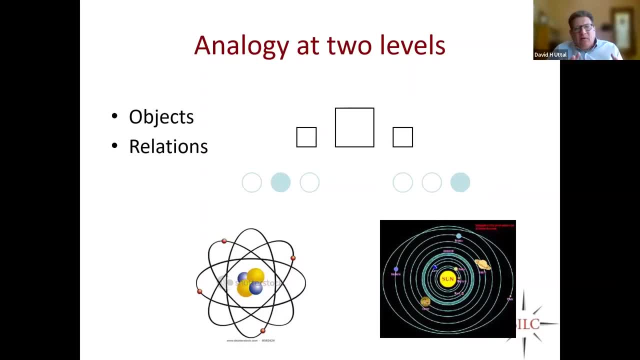 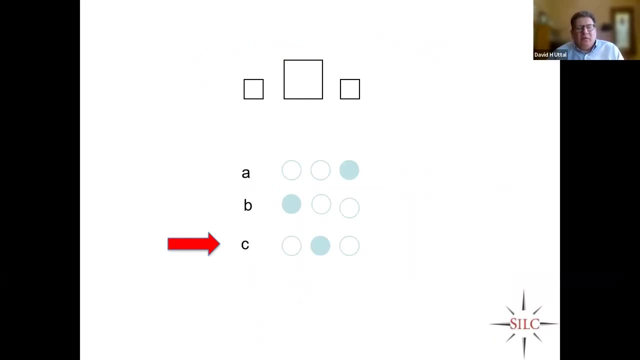 objects- i'm going to go quickly because i think most of you know this, but it's important- objects and relations. so objects are the things that you're reasoning about: squares, circles, electrons, planets, whatever it might be- and relational structure preserves how objects are related, even if those objects are changed. so, similar to the first example, most people have no. 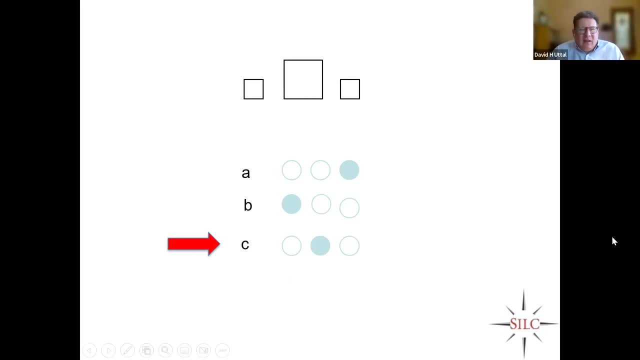 trouble if i say which of these three i gave the answer away. so it's not going to be a very entertaining quiz, but most people would not have trouble picking. c is the correct answer, even though everything- obviously the object property pretty much- is different. it's about circles versus squares. it's using patterns. 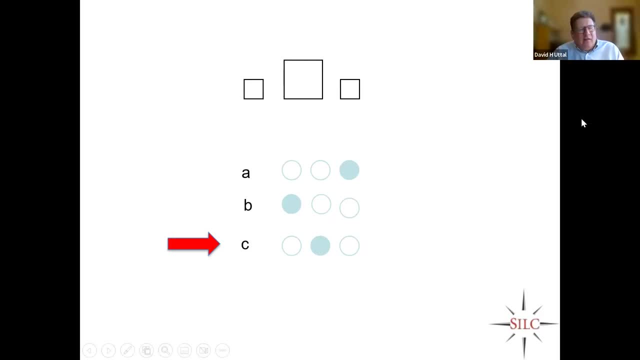 of shading or fill or color versus size and all of those things, all those object properties, are irrelevant to solving the problem. and the fact that we can do this and other species struggle so much is, i think, our, you know, evidence of our relational status. uh, it's interesting, the um. 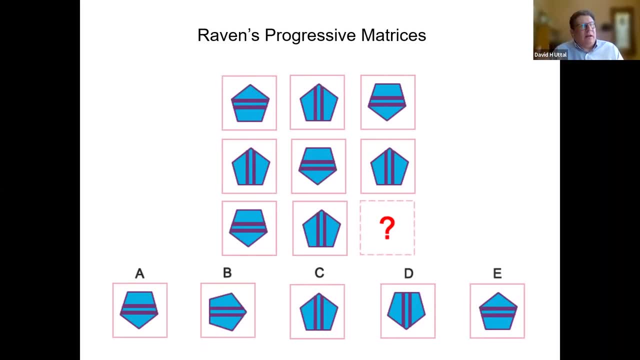 forbes, andrew, um, i can't remember. i'm sorry if you're here i can't remember your last name, but several other people have modeled, uh, the raven's progressive matrix, which is often seen as sort of like the single, the, the test of intelligence that correlates. 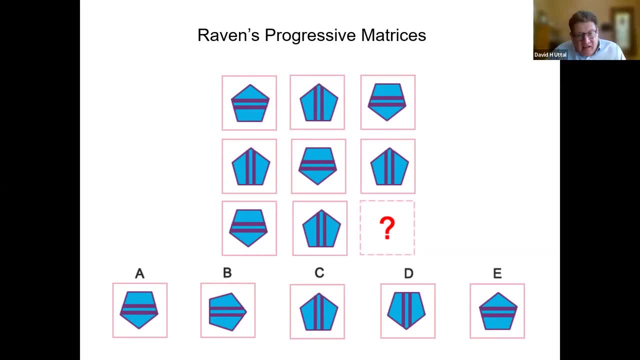 best with all other tests, um, and it can be, in that we know this both empirically and computationally, that it can be thought of as a relational mapping task, and so, again, it is both a spatial task and a relational mapping task, and this could be thought. 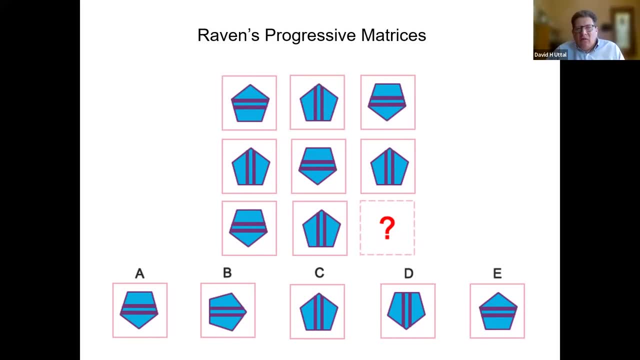 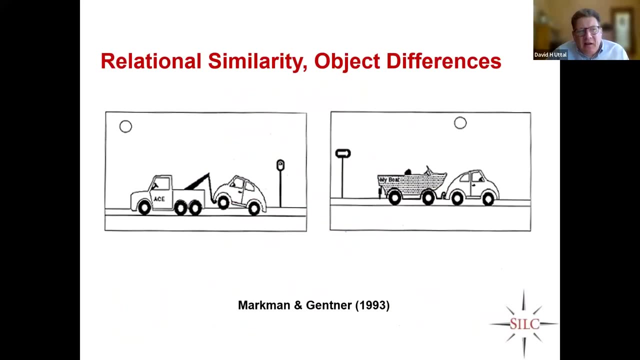 of as your ability to take all that the universal donor can give you and solve these problems. okay, now, one of the things that comes out of this theory is we can have mismatches between relations and objects. in this case, the relation is the same- the pulling- but the puller and pulley have been changed. it looks a little odd. it might be a little bit. 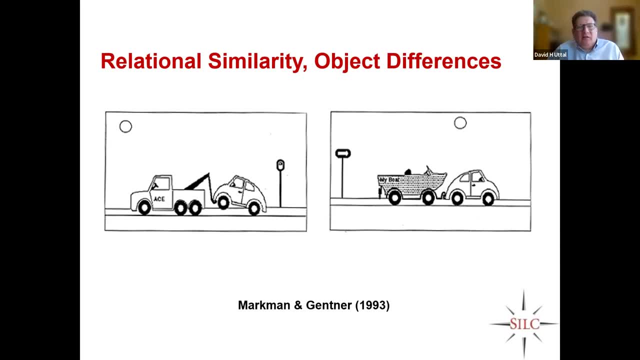 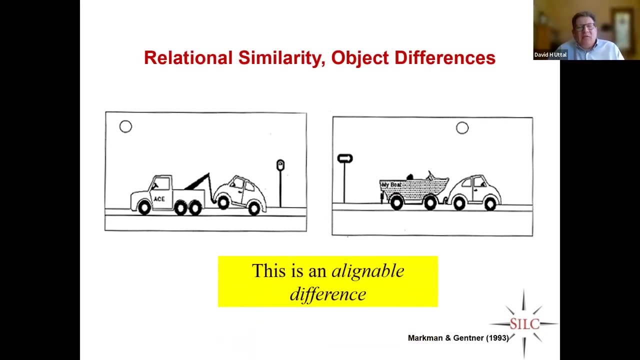 troubling to a young child, but the basic idea is pretty clear. okay, i understand it. the volkswagen beetle is being towed in one case and is the tower in the other case, but the relational structure is clear. um, and we call this an alignable difference because the difference emerges from: 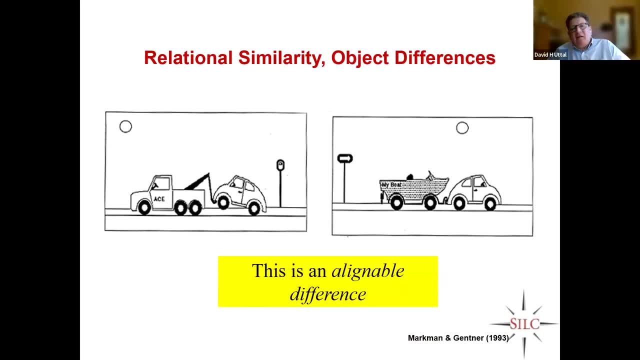 the alignment. so it's relations first and then we pick up a difference. So sometimes things are seen as different that are actually very related. Hotel and motel is an example. You can come up with a lot of differences between those, but at some great surface, object level. 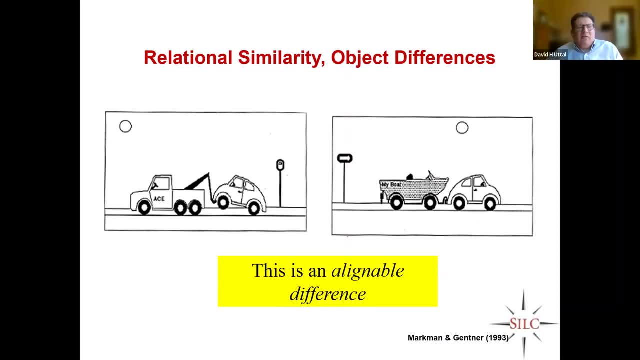 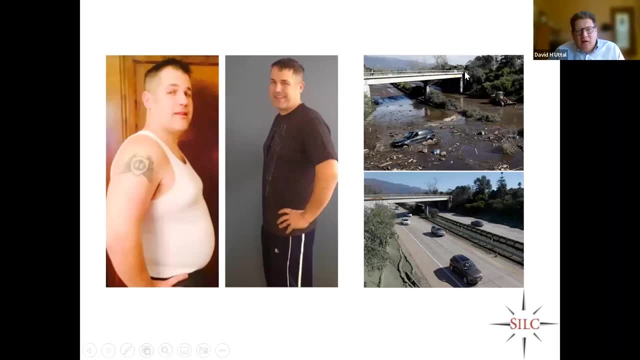 they're very similar, but it just shows you how prominent relational thinking is And we can use it in other examples. This is actually a real California flood and when you see the difference, I don't know why. before it's below, but before and after. 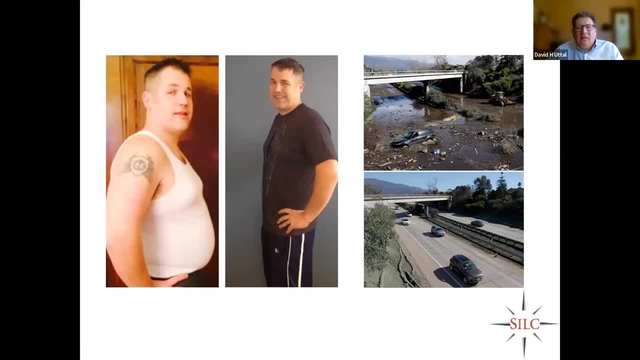 it really drives home the difference because the relational structure is the same. You can barely pick it out, but this bridge, fortunately, is still standing. Nothing else is That relational structure makes us really notice the difference And likewise one of the reasons I think that 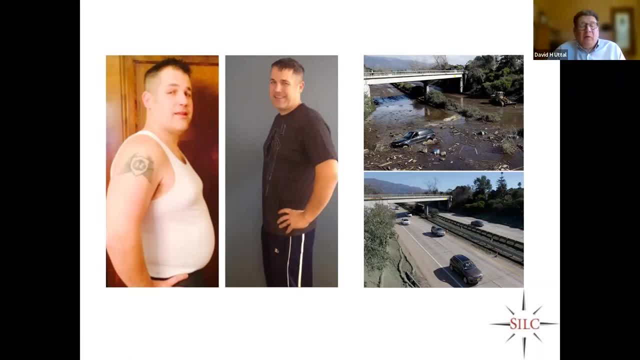 before and after pictures are so popular is they create this alignable difference. It's the same person, but the physical difference really pops out when you align the two, And so I think there's a reason we're so obsessed with these before and after pictures. 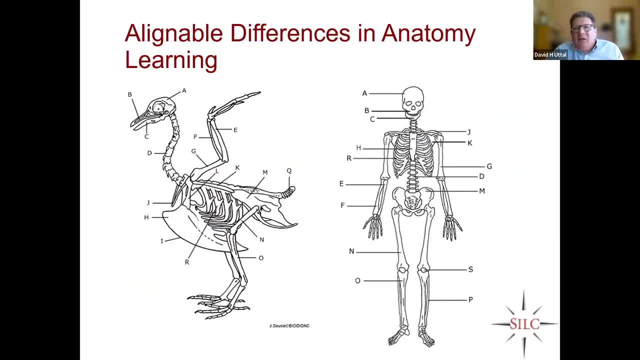 Okay, And then many people: Brian Matlin, I saw on here. there's several other people, Kurt, I'm having some trouble with names, but in any case, many people have worked on this problem of applying the universal donor of spatial skills and alignment to science learning. So this task. 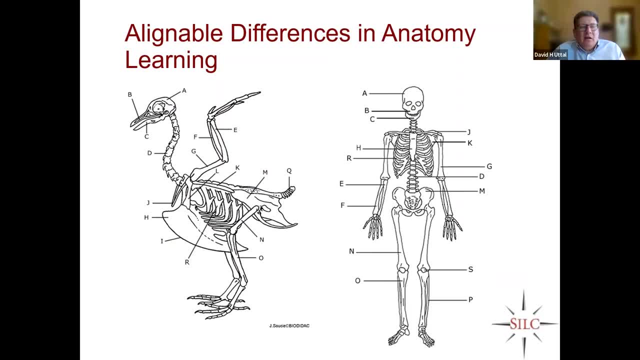 is for students to pick out structural similarities between things that look kind of different to start with. So we share a commonality between the two And I think that's really important And I think we should talk about this. but one of the things I would like to sort of look at here is: are the 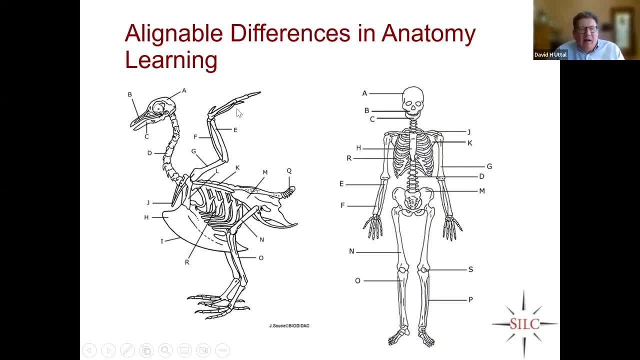 two uses. the very first, of the neighbors to the social mencionations, I would like to start out with 가장 important here. The first of these people is the spatial visualization and the relational thinking. Okay, and so relational, I can't read the top of. 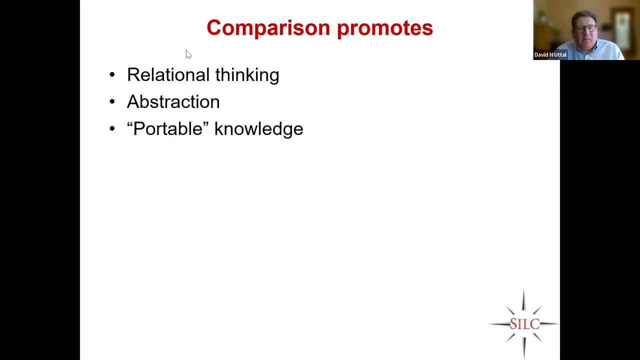 my slide. So when we do this kind of comparison, it promotes the relational thinking, also abstraction and portable knowledge. that we can now think about skeletal properties rather than about individual bones is one example. We can think about relations like middle, despite the individual properties, like two and four, there's a middle between them. four and eight, there's a. 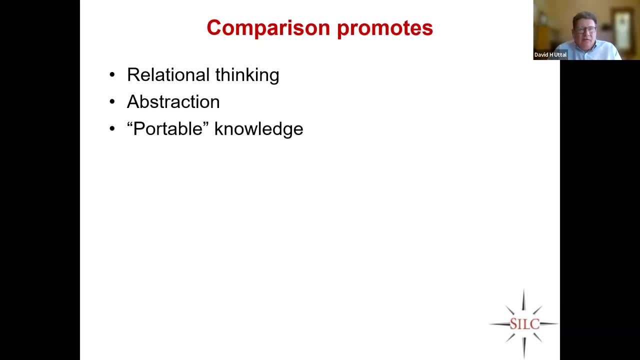 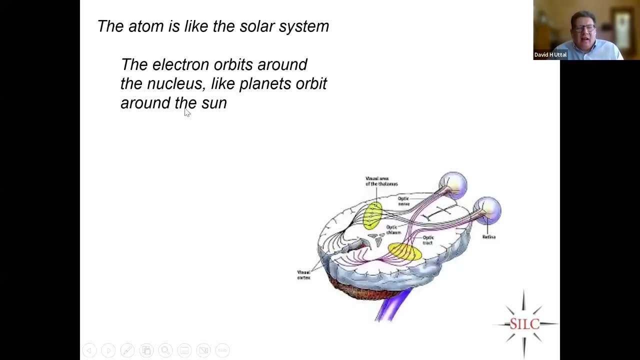 middle between them. Those are different numbers, but we still understand the concept. Okay, so at a psychological level, what I'm saying is that we are- and this is pretty well documented through MRI and things- we're taking advantage of some of the properties of the visual system to briefly visualize relational information. 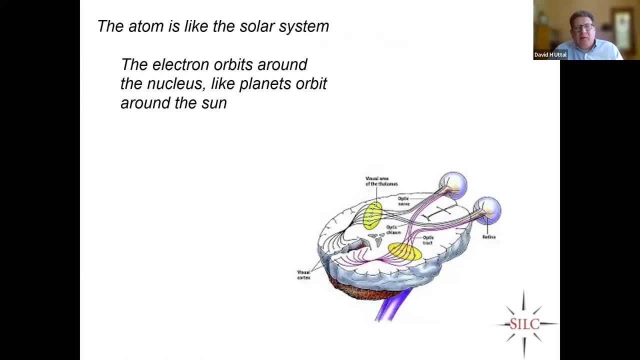 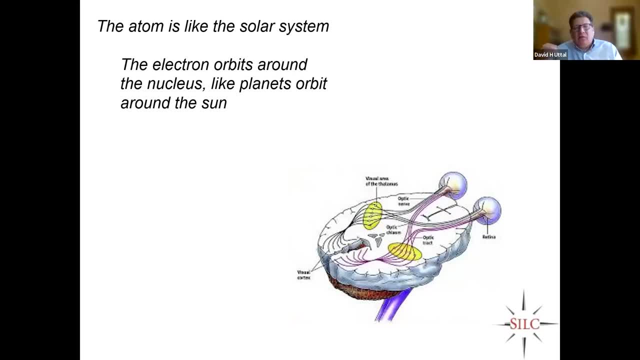 it's limited and we have to construct a visual representation purely from linguistic description is quite hard and requires a lot of memory. We can do it, but if you're faced with that task, one of the first things you want to do is restrict the amount. 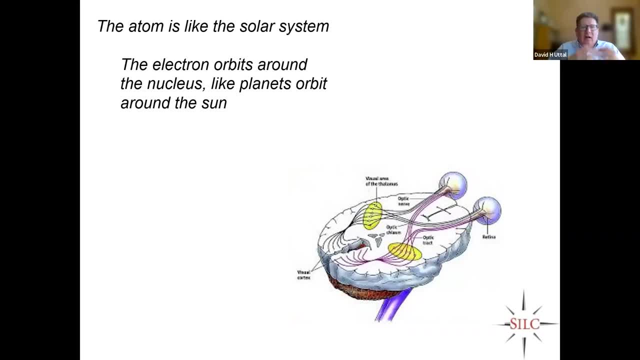 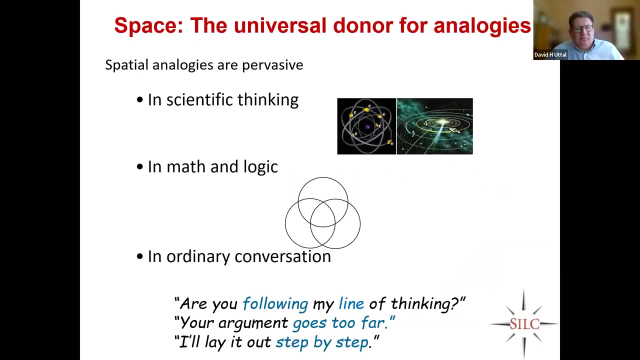 of information and or get a piece of paper where you can now take advantage of the universal donor and think visually. But in both cases we're sort of using some of the properties of the visual system. Okay, So I, you know, made the case that space is the- or I'm sort of developing. 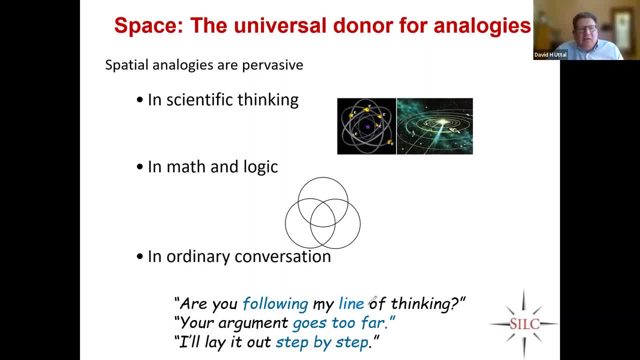 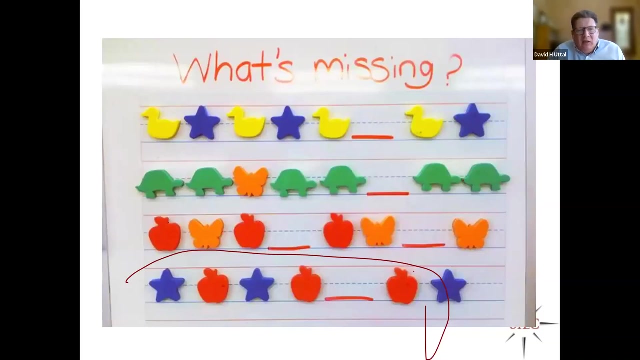 Dedry's case, And you could see it not only in STEM but in everyday thinking. I want to make sure I get through, So I'm going to advance on. I do not want to color. Wow, I am caught in this. Okay, I think I escaped, Okay. So now let's talk a little bit about early mathematical. 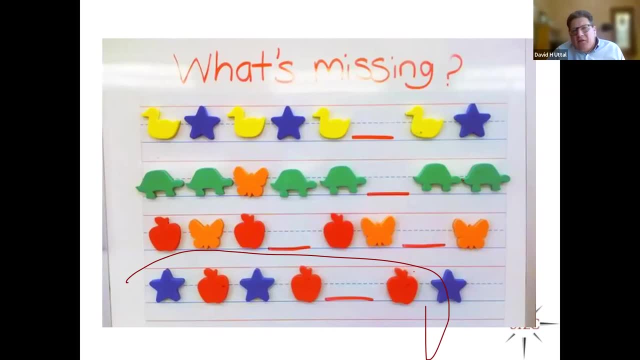 development. I noticed that Bethany Riddle Johnson was a member of this group. I don't know if she's on, but this is based in part on on her research on the value of patterning for learning early mathematical information. I remember a quote. I can't remember who said it. 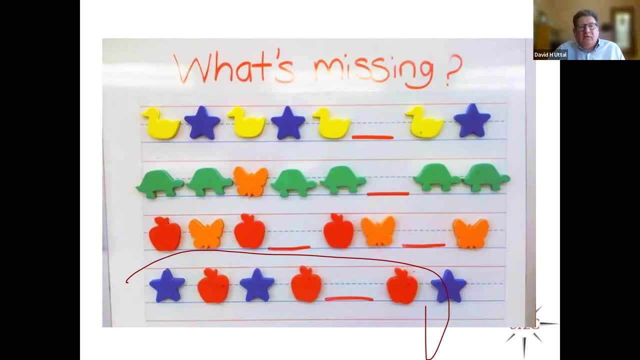 but it's like every good kindergarten teacher knows the value of patterning. Now, there's not specific numbers assigned here, but you can. you can do that, or symbols, AAB or something like that, or ABA or whatever it might be. But what's so important here is it's about relations, very simple relations, but some kind. 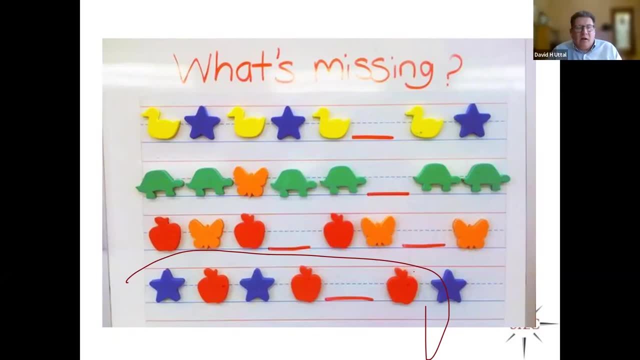 of relation between the duck and the star or the turtles and the butterfly, And it's in those two top lines. it's depicting Two different kinds of relations And it seems- this is a summary of a great deal of research- that patterning is predictive of math skills. About two years later, two or three years later, 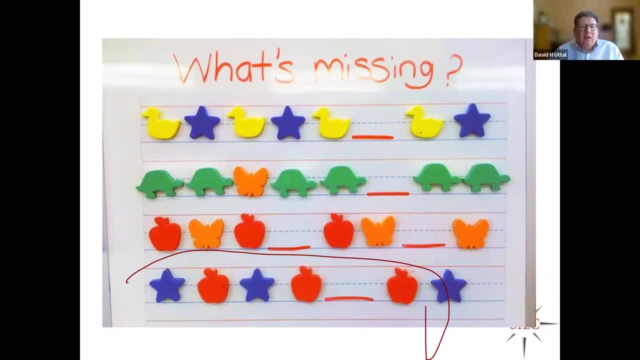 and, moreover, it can be taught, And I think what we should think about what's happening here in part, is we may be facilitating students thinking about relations, not simply about apples or butterflies or turtles or ducks, but about relations, And I think that's a great way to 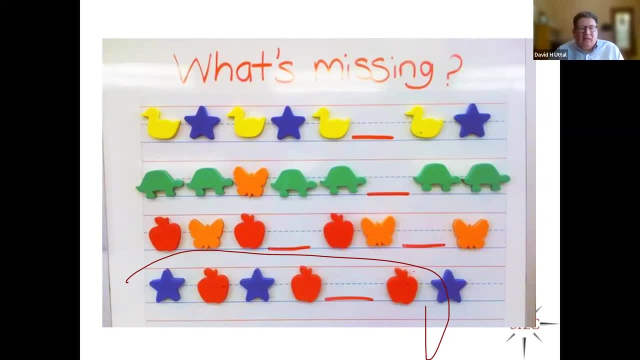 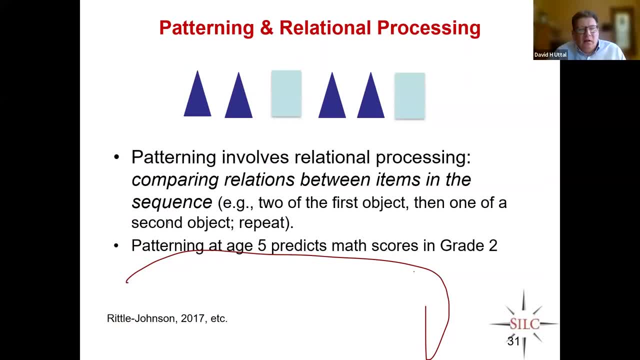 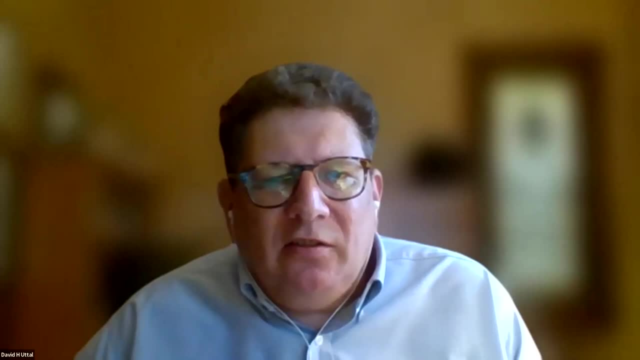 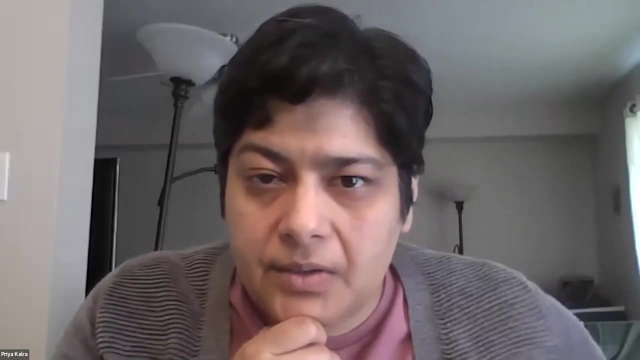 So this is from Bethany's work, explicitly saying that patterning involves relational processing. I would like to try to get rid of this red line. Did I? Okay, I shouldn't try too much. Okay, I think if you restart the slideshow, that could work. The other thing is, I think there's an icon. 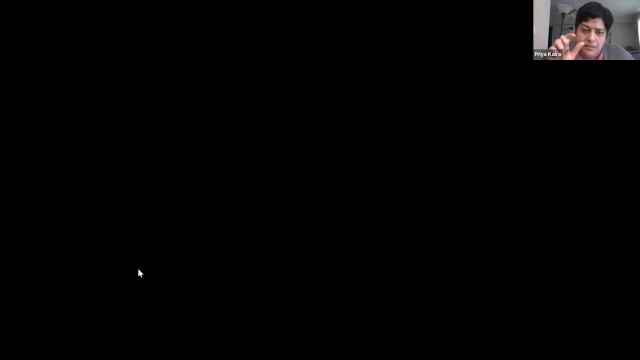 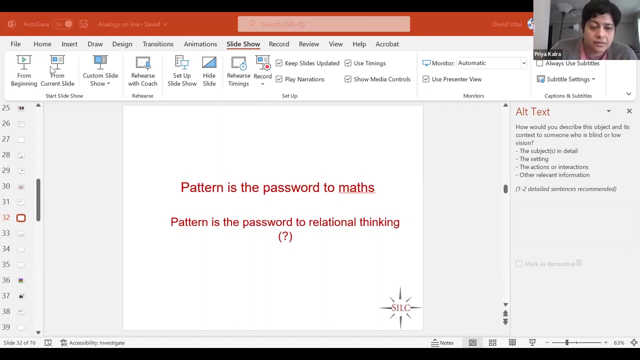 in the bottom left for your cursor And you may see an eraser there. if anybody else, I'm just using the very crude first method of restarting That works. Your second one is very elegant, but I like that. So somewhere, somebody, it was someone British. 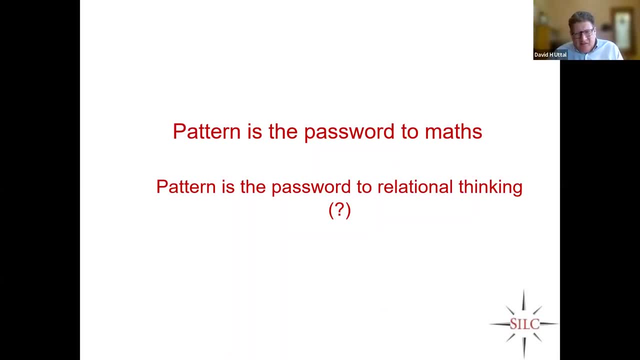 because they use math plural and Americans tend to say just singular. But another quote that I can no longer attribute, floating out in the ether there is: pattern is the password to math, And which I would then translate pattern as password to relational thinking, and relational thinking is important for math. 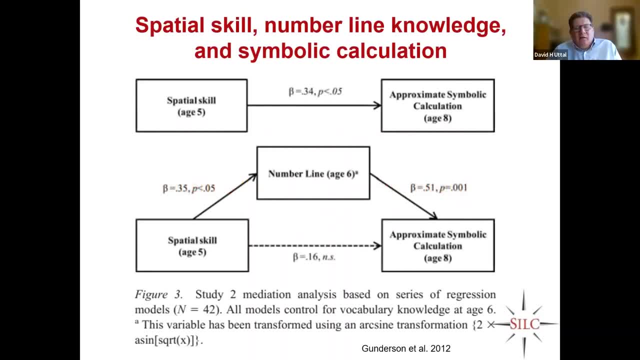 So let's talk a little bit about the number line. So some of the one of the things that's happened in the past 10 to 15 years is we're starting to move beyond just simple correlations between spatial skill And STEM learning to much better understanding of how, when and why. that's true. 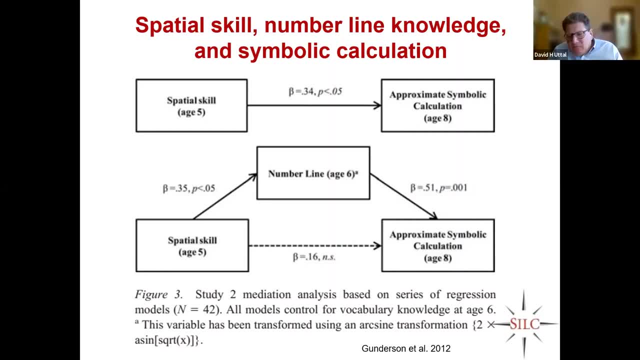 Mostly in early math learning there are some continuations, but one of the nice things that's happened is the alignment between all the research that's gone on in number learning and in spatial learning have kind of come together to give us some insight into what is actually. 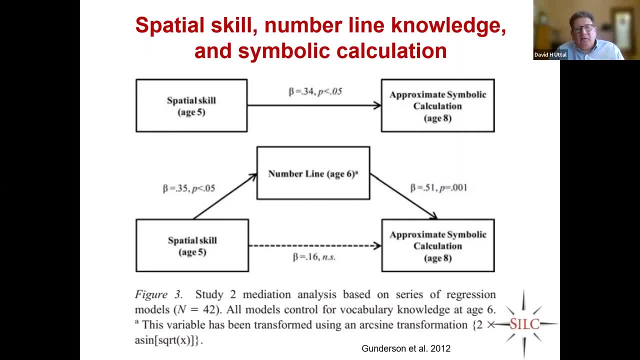 happening when children learn about numbers, And for the first thing is there's a lot to learn. Yes, we know from Spelke and others work that we are born with some very important numerical skills but, importantly, they don't give us all that. we need to learn math. We have to map on what we hear. 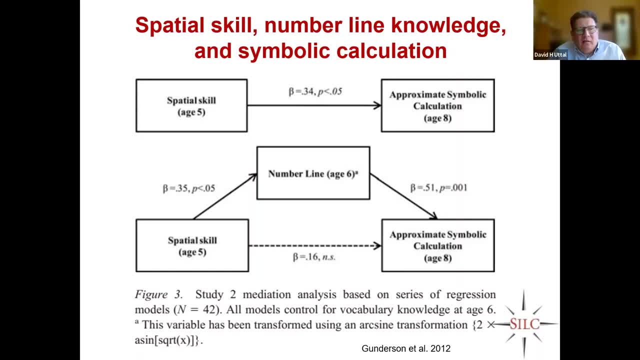 number words, for example, to the linear nature of integers. That seems to be a very important insight. Number sense: understanding how numbers increase with increasing quantity and how they're related to one another. This is work by Elizabeth Gunderson and team in which she looked at spatial language and number. 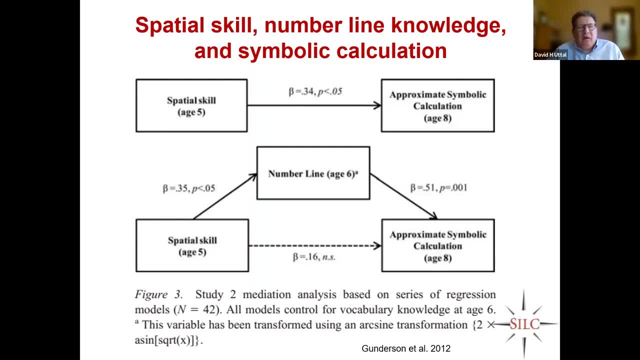 line skill and approximate symbolic calculation. years later- And this is interesting because this is a naturalistic study- They went to the home multiple times. This is not an experiment. They did nothing to create the variance that they observed. This is naturally occurring variability. And then they use linear causal models to try to 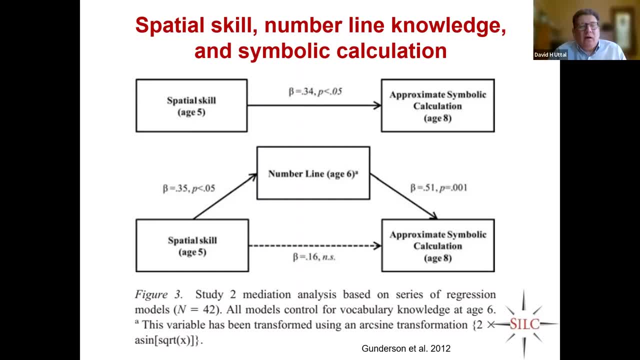 take out variants that might be due to things that are less interesting. The first thing is that spatial skill, as measured at 85, does predict approximate symbolic calculation where you're asked to add numbers and see how close you can come. But that relationship is mediated by number line knowledge. So if we, if we look at number line, 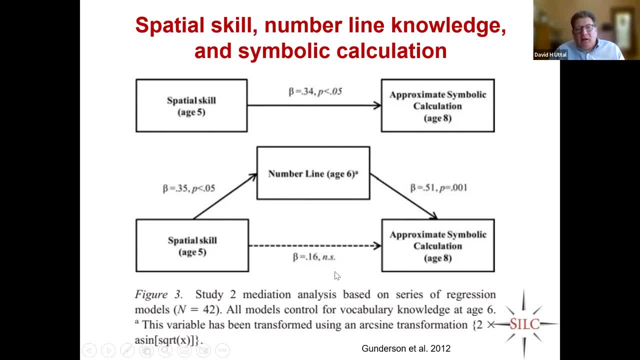 knowledge. we don't have the number of water that's going to hold the ident Bremen Columbus knowledge, that absolute correlation here becomes non-significant. This is just classic mediation, So that the variance between spatial skill and approximate symbolic characteristic is largely explained by number line knowledge. And why is that so? Well, I think the number 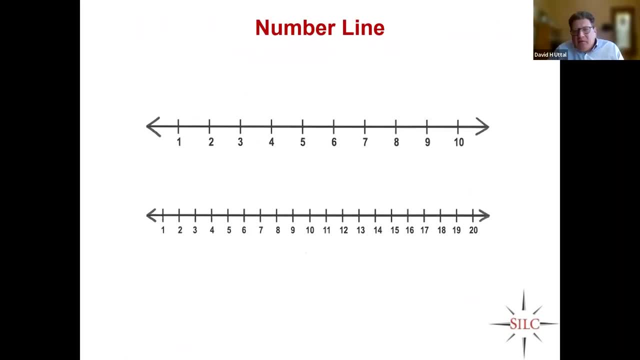 line is one of the first spatial representations, be it only in one dimension. but the universal donor is starting to give away information about relations between numbers. So there's debates about what's learned first, and can you have relations early on without knowing the individual? 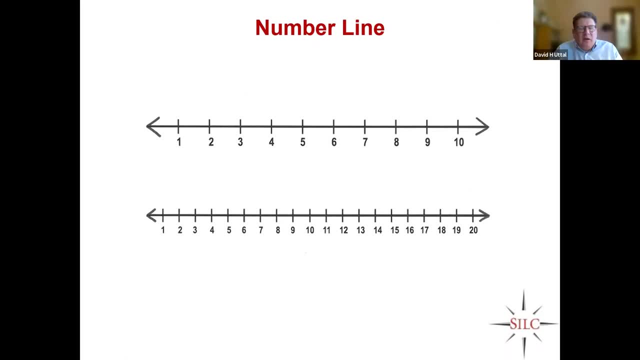 facts And I think there's huge debates about all that that I'm just waving my hands both literally and figuratively at And it's really important. But it seems to me that one of the things that you get out of the number line and why it's so important is how and why that these are related. 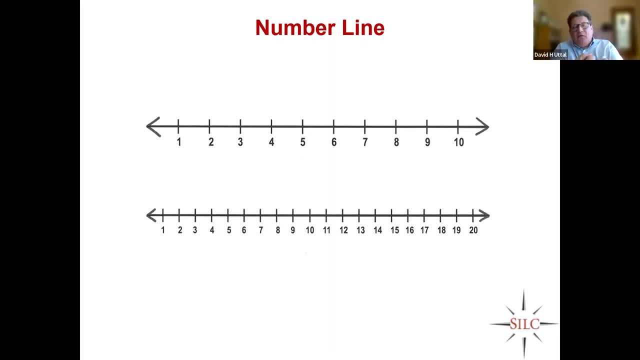 that there's increments by one and then that maps on to an increasing distance in a constant way. So that's absolutely critical information that you don't get simply from counting. So this is why we have two knowers and three knowers and lots of people, lots of kids, knowing certain numbers but not knowing how they're related. 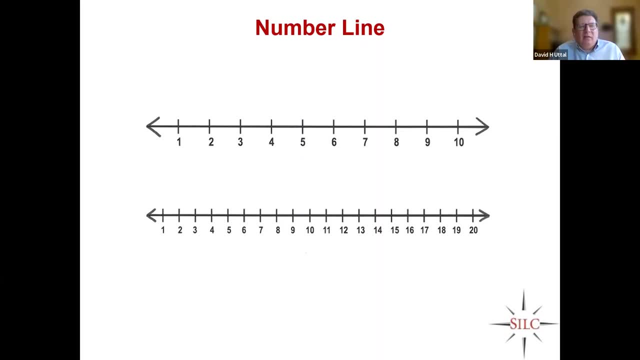 And the number line seems to be critically important to understanding that. Part of that is literally learning about the number line And some of it is acquiring a mental, mental number line. Good spatial representations- simple, elegant ones like the number line- help us to internalize them. So it's become a tool for thought. but it might well start with 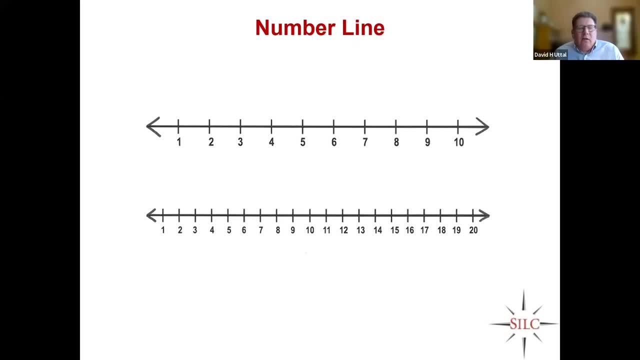 the external representation and the mapping of that onto the number words that they hear. So this is a critical thing. I think Susan Carey- I think she calls it- something miraculous happens. It is miraculous, but it's also perhaps somewhat the miraculous event is to map. 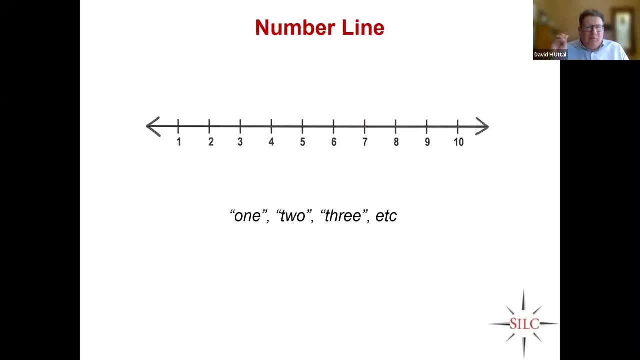 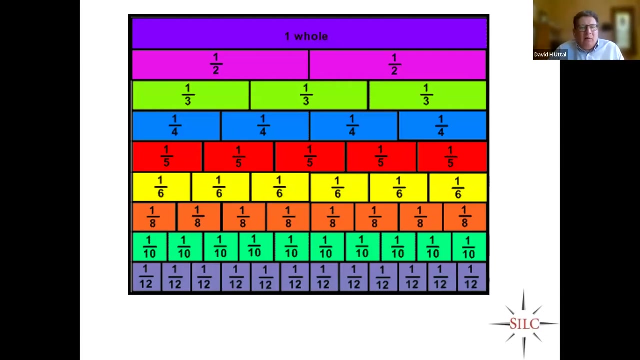 on increases that you hear in words, to increasing quality. It's not easy, but I think that the spatial mapping gives us a critical foothold into that relationship that we can then build on. Same with fractions: number lines work and seem to help in fraction two, because 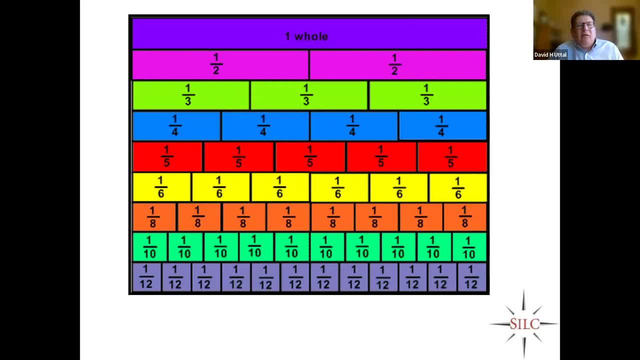 what children have terrible time with is understanding the relational nature of fractions, And they'll often say: one third is greater than one third, And so you know one third is greater than one third, And so you know one third is greater than one third, And so. 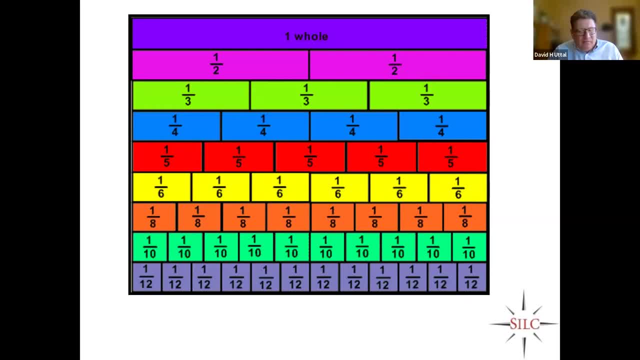 one third is greater than one third, And so you know one third is greater than one third And so than one half, because three is greater than two. that's incredibly common error and also, uh, this is like the second great roadblock to learning mathematics. so the first one is number sense. if 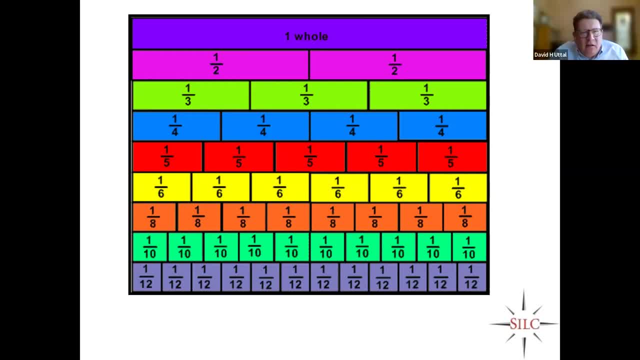 you don't get over that, you're in bad trouble. but then fractions, um, it seems like every other grant proposal that i read, you know, when i was on the panel- was: american children are really bad at fractions and fractions are really important for the rest of their lives. and it seems like 50 of 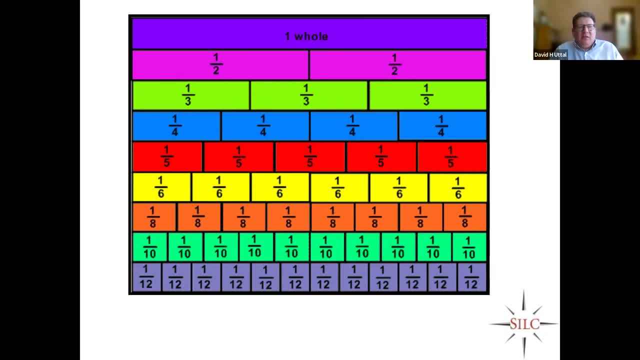 the grant proposals have that basic introduction which shows how important the problem is uh. number two, that no one's been able to solve it yet. but number three: they have some intriguing ideas to do so and a lot of it is about seeing uh relations amongst numbers. this is conveying. 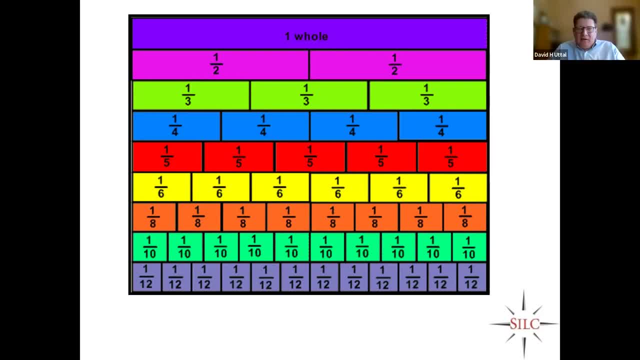 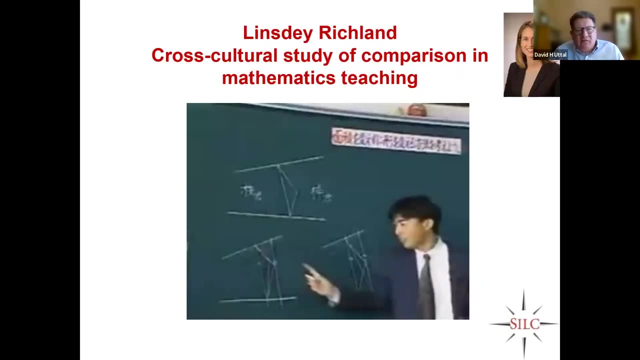 a relational understanding, and then we hope that either the teacher or the child on their own will map the numbers onto the partitions. and that's the fundamental insight. we know that um analogy is used in many learning circumstances. lindsay, richland and colleagues have shown how important uh interesting differences between how analogy is used in japan and the united states. 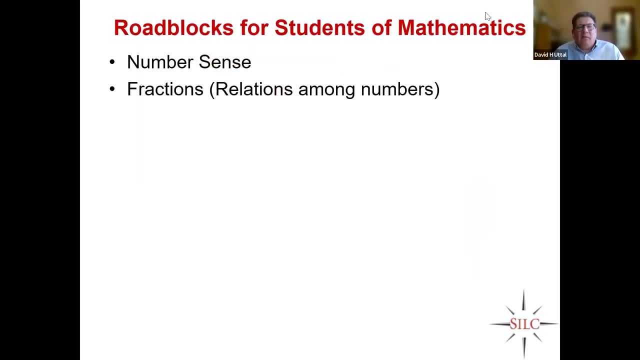 um. so let's just end this part by um, looking at some of the most fundamental roadblocks for learning and mathematics. i've already talked about two number sense and fractions. the next one, accounting for the other 50 of the grand proposals, is algebra um. this used to be, you know, considered a sort of a traditional eighth grade. 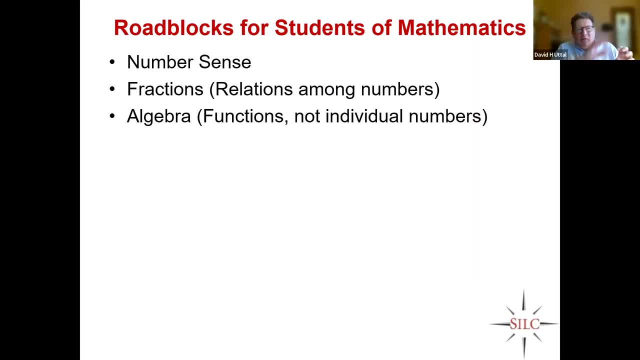 problem now. there's attempts to introduce it much earlier, embedded within the curriculum, but seems like a lot of students really have difficulty making that algebraic length, and this is critical, because now you're taking math as a symbolic language, and that's one of the things that math is really good for. so functions. allow us to think about relations. 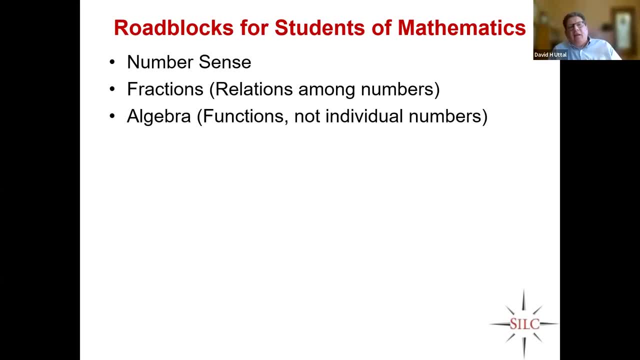 amongst numbers and and they apply across any individual number, and that that is definitely a relational understanding. and then finally, calculus, which is one that you know, i'd say most students you know eventually get these, but then calculus is kind of it does distinguish people, who who go on in stem versus versus those who don't. so high school calculus has become. 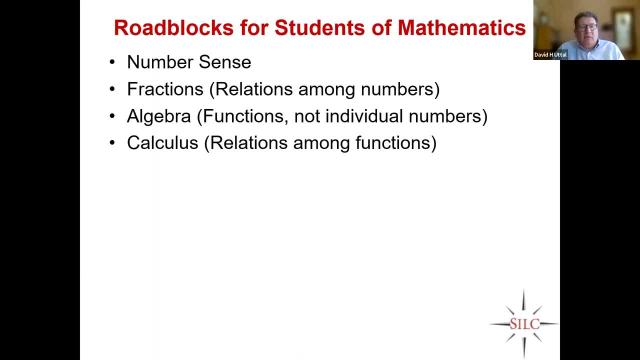 very, very important for predicting who goes into engineering, for example, and that is about relations amongst different functions. so just defining what's being looked at, learn mathematically, rest upon what is being related to what, and so it seems you know. obviously this is just completely correlational, but it does suggest that when we're changing what the relations are about, 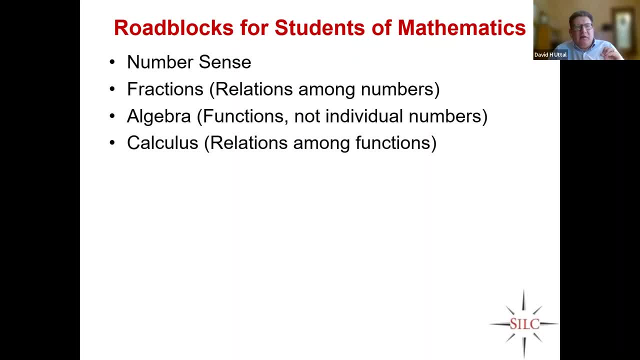 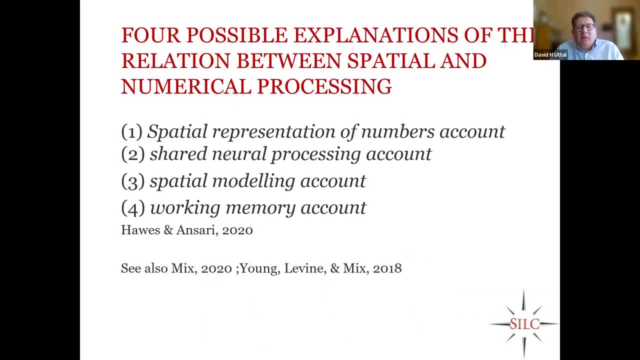 children do seem to be particularly at risk for not catching on, and maybe some of our instruction can can help in that regard. you okay, now i'm going to very quickly consider um some recent, a recent paper by uh haas, zach haas and daniel ansari, um about why math and space are related, and i'm going to do this. 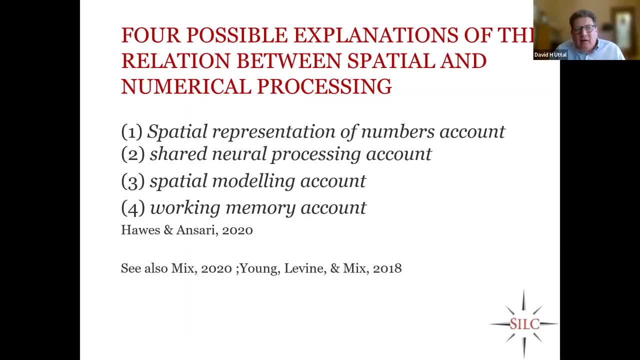 quickly. but i want to say that the basic argument i'm making is that each of their four possible accounts really have to do something about relational thinking, that although they don't ever come out and directly say that it looks like in the making, i think you can read their paper as saying that. so 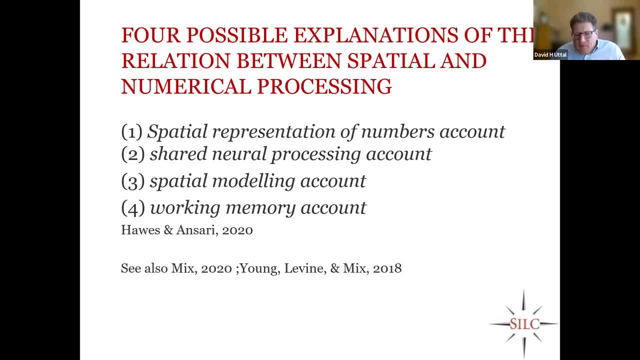 to be fair, this is my interpretation of their paper and i should also point out that many people working this particularly kelly mix, sometimes uh alone and sometimes in collaboration with haas- are working on this um in detail to try to understand why math and space are related. 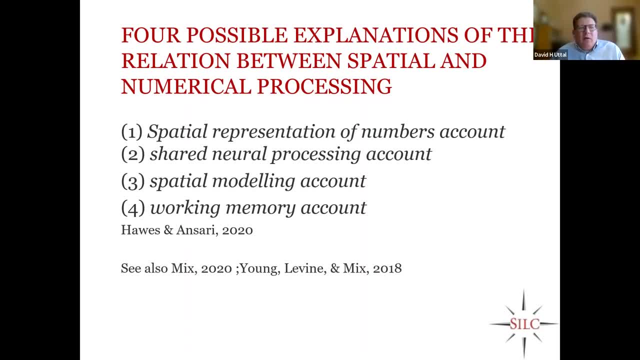 and, of course, i think it's like really important and i'm like hoping we're all converging, okay. spatial representation of numbers account. that's not just typing um we– its actually the боль of space as well, which is, uh, one of the levels that has started to change themath and spacegenics. 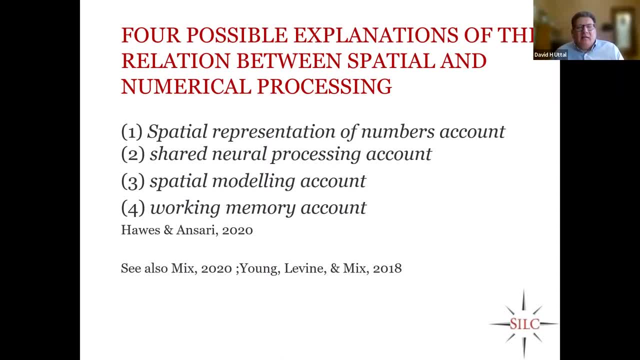 space Disneyland. all right now. all we need to to. In some cases we already know w hat. if y'all read aren't expecting basically the number line, They're saying that you know what I've already said: that space outlines relations amongst the numbers Shared neural processing. there does seem to be specific. 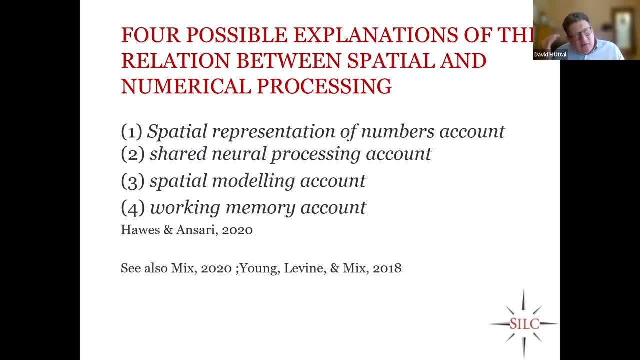 brain areas, one of the sulci of the parietal cortex that seems to be stimulated or used more to to share, to certain kinds of math problems and certain kinds of spatial problems. Spatial modeling is in some ways what I've talked about the most, which is that we construct a model. 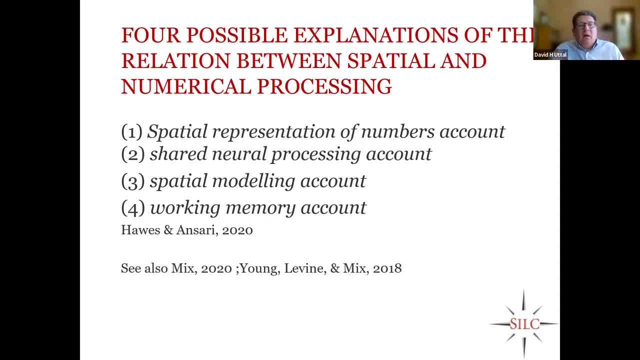 be it either physical, on paper or in our mind. that allows us to think about the mathematical relations. Now that number three is basically my favorite approach, although they they say that these three are not, these four are not in competition And working memory, that it reduces working memory, and that's certainly true. but importantly, 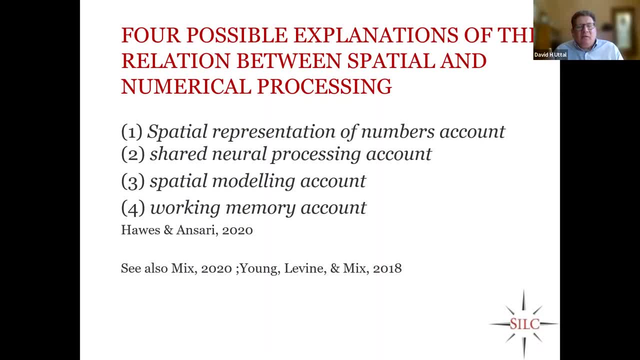 working memory reduction works best when most efficient, when we can apply relational structure to it and not just a limit like this is one of the reasons. like straight up working memory training doesn't seem to transfer, because using our working memory is smarter than that We try. 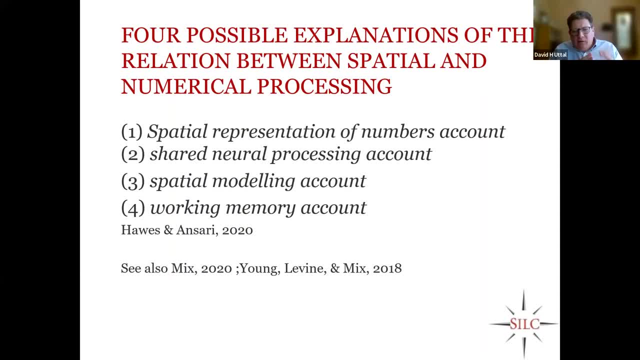 to look for patterns and relations So you can train working memory. but it doesn't seem to transfer, And so I think that's one of the reasons why we're, But it's been hard in a general way to make it transfer to other things. 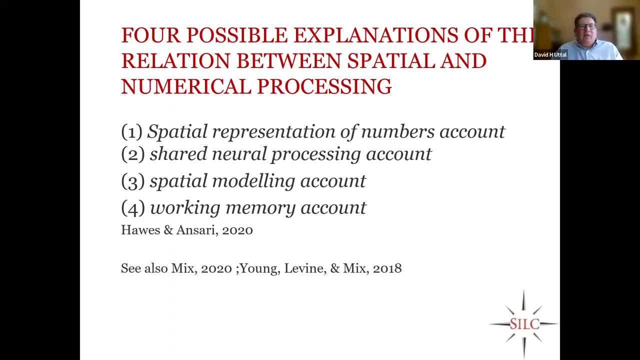 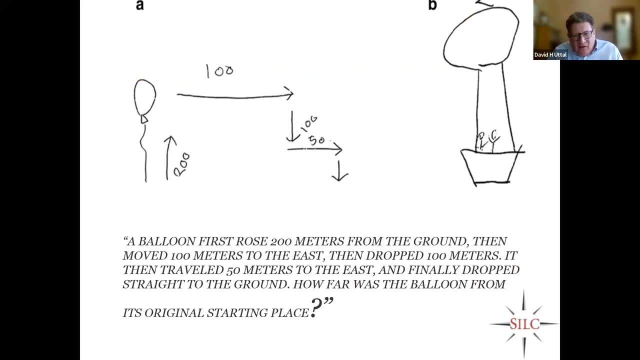 But I think that's a misunderstanding of how we use working memory. So I don't disagree with any of these. I think what I'm basically saying is number three might be the sort of number most important. Now, this is my interpretation of Hans and Ansari's interpretation of a study by Hegarty. 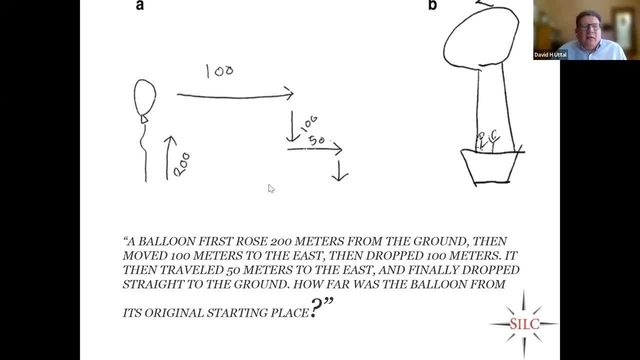 and Maria Koskonica that they did in 1999, where they gave children math problems and then provided paper but didn't tell them what to do with the paper. I think they might have said, like drawing a picture can help, or something like that. 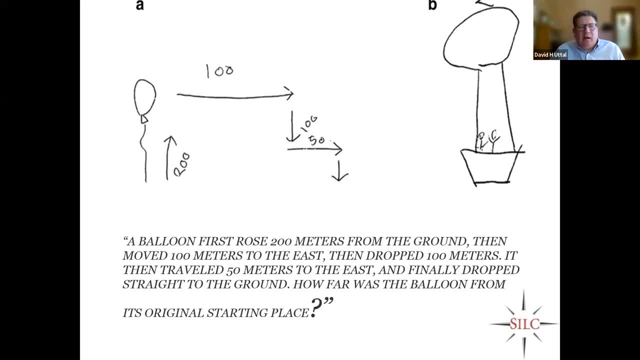 So there are problems like this: A balloon first rose 200 meters from the ground, then moved 100 meters to the east, then dropped 100 meters. It then traveled 50 meters to the east and finally dropped straight to the ground. How far was the balloon? 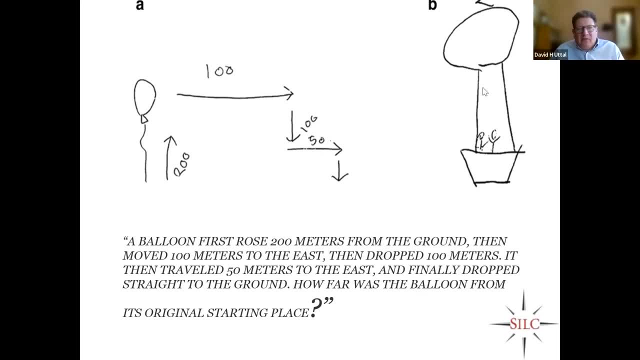 How far was the balloon from the ground when it started? Some kids draw pictures. This is the graph as picture notion. It's basically a narrative. It doesn't tell you anything. to solve the math problem. Others do something like this And I think this is a really good example of spatial 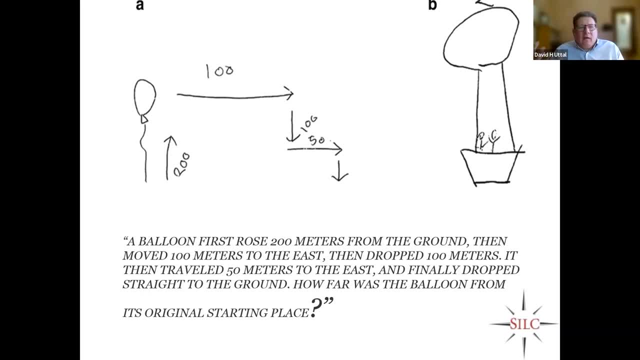 I think there's a reason that drawing the arrows. arrows are about relationships between direction and force or distance, And They could simply list the numbers, you know. but there's a reason: as a transition from the physical, actual things that happen to more of a relational structure that comes 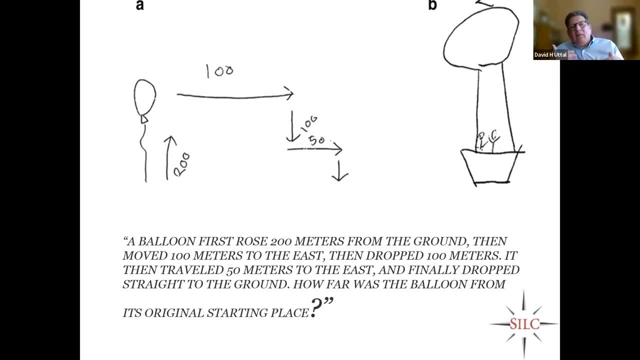 out because of the spatial modeling. So we can have a long debate about just how important is the spatial representation to solving this. I could see it all the way from critically important to just almost like an epiphenomenon. It's just making the child write out the right numbers. 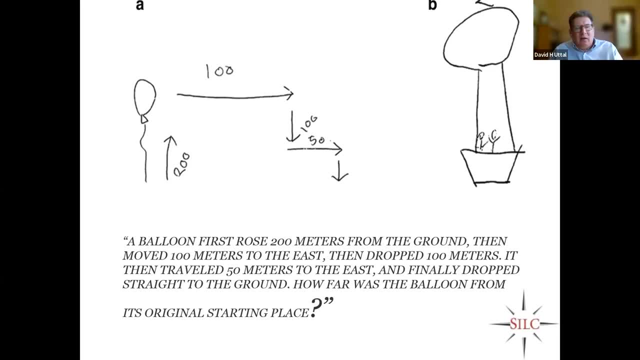 Even if it's only that last one, that's still important, but I think it actually is much more than that, And that they're- they're imagining it traveling to space and then assigning a number and then thinking about how that number has to relate to the next number. 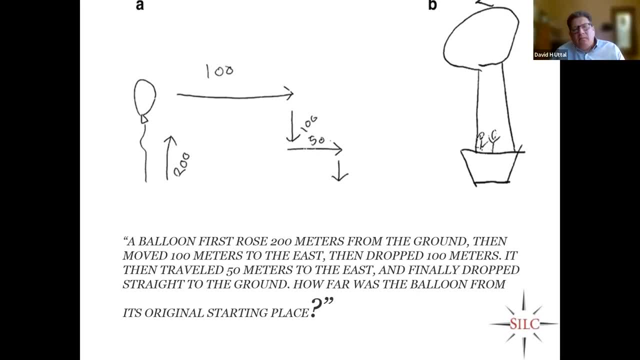 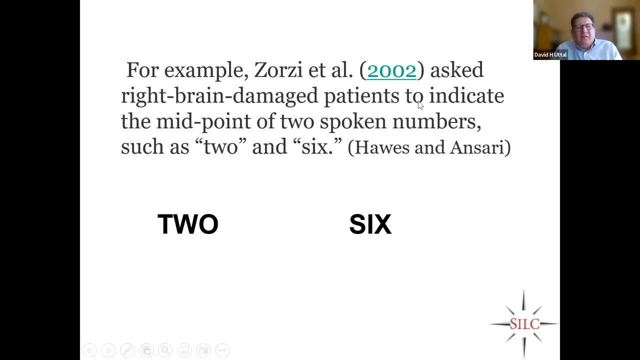 So the spatial modeling is part of the numerical problem solving in my mind. Okay, Another example that Haas and Ansari site is in some brain damage. They seem to have a non-relational understanding of between this or middle. So if I say, draw a midpoint between two and six, it's easy. 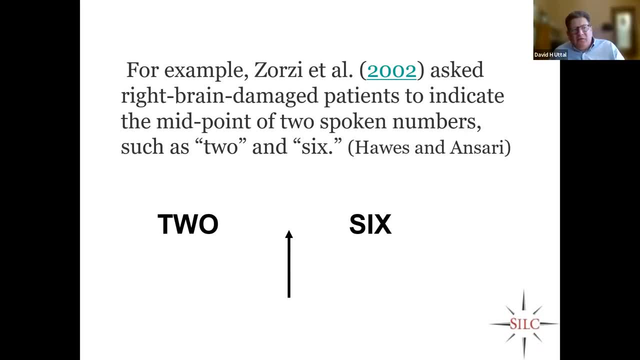 And I, as long as I keep it proportional on the two sides, the two numbers, it's going to be the same place. But in this, in these patients with parietal right brain damage, they are more influenced by the larger number. 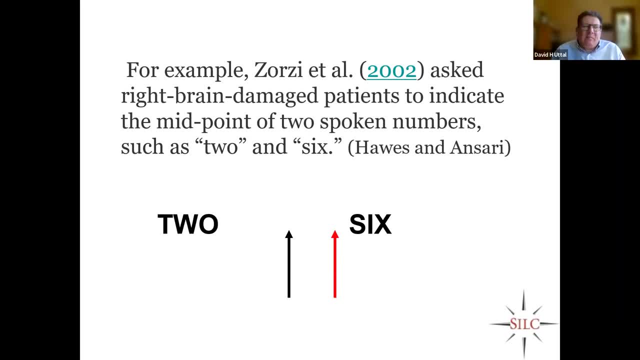 So they know, they seem to know what has to be somewhere between. So they understand Between this but not middleness. in a way, in an interesting way, And that is exactly a relational understanding- is that the middle is, or midpoint is, based. 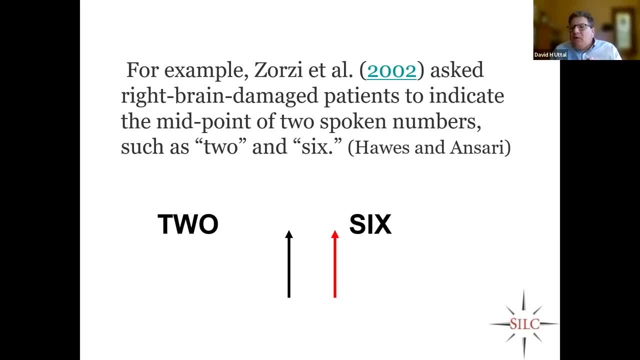 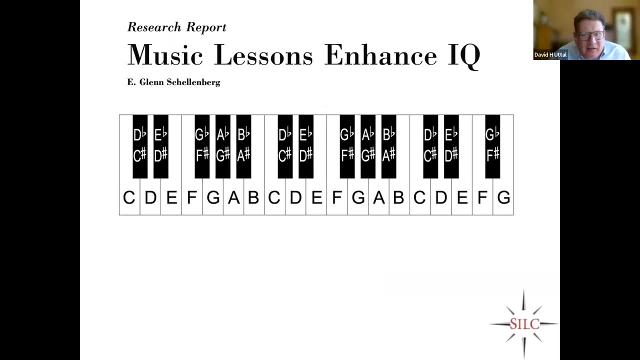 upon the relation between the two, And this is a difficulty in mapping space back toward number. So it works both ways And I thought this separation again shows just how important the relational understanding is. Okay, Now, this is the most speculative. I couldn't resist putting it in, and I know okay. 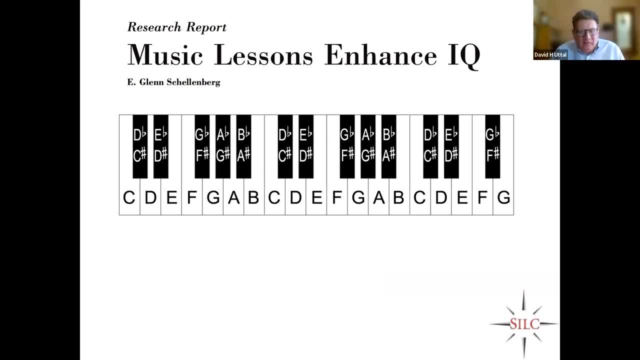 Even saying there's any relationship from music lessons in an IQ is very controversial. First of all, I'm not talking about the Mozart effect, where you play Mozart and then they do better on spatial ability. That's specifically that has a mean effect size of zero. 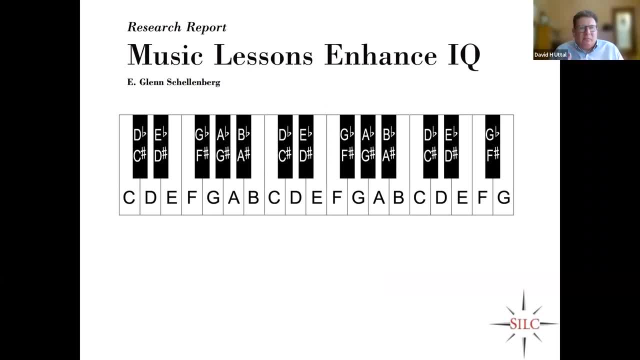 It's just, it was a odd finding that was published. Meta-analysis showed that it was, that it was an odd finding, but I hear I'm talking about learning about structures, Structures and patterns and relations And in this regard we've wondered sometimes: are some instruments going to make this pattern? 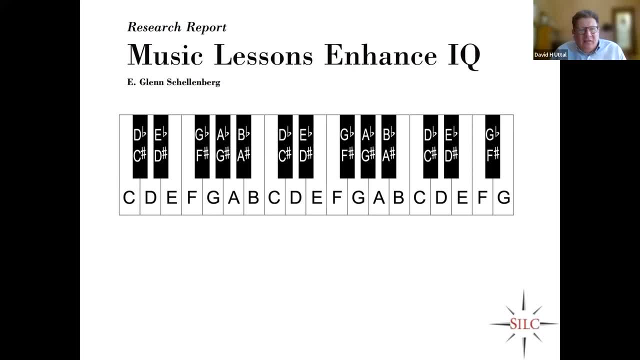 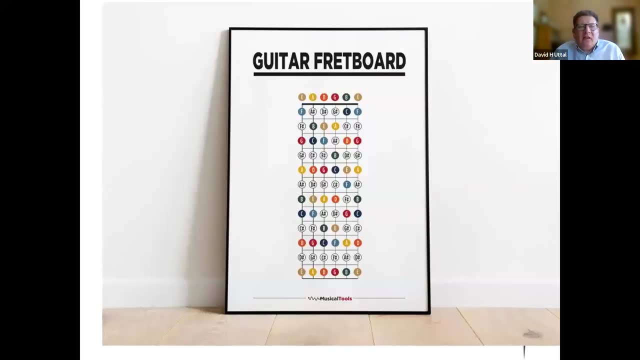 easier to see than others. I think that keyboards actually, you know, replicate a pattern And this is something I've never seen, tested. but I would love to see how music lessons affect IQ in for different instruments. So a guitar is an interesting contrast and I'm, as I've been, struggling to learn myself. 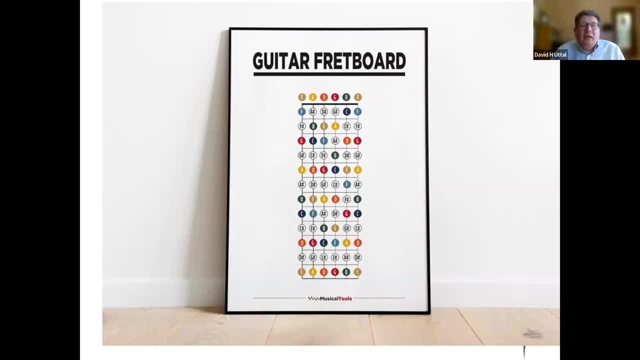 the patterns are there, but boy, they're hard to find. There's nothing about the guitar itself that tells you that it's the length of the strings that matters, because they all appear pretty much the same length And they certainly look that way at the first fret. 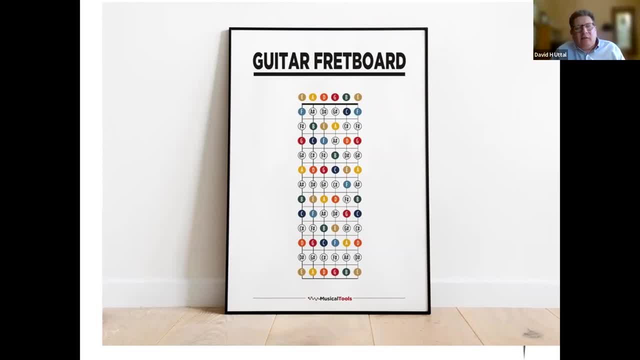 If you understand the engineering of it, you could get some insight that it's string length, but also, the first thing they teach you is basically where to put your fingers down to make different sounds, which doesn't tell you hardly anything about the relation. 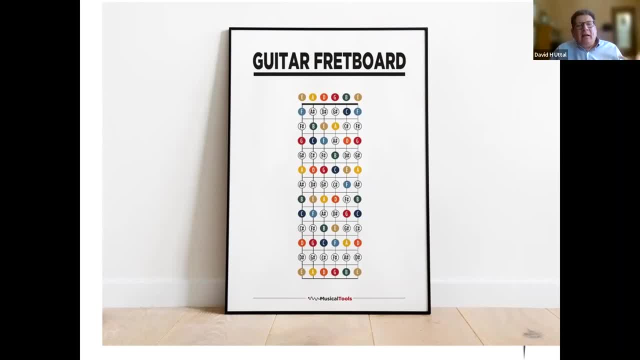 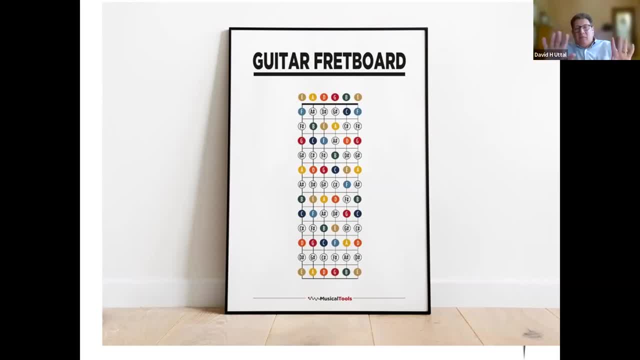 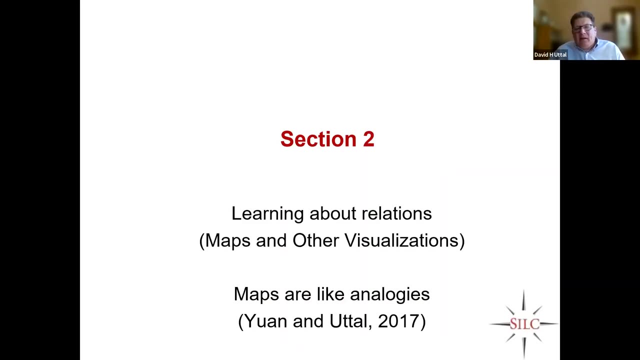 to me just less apparent. Now, some guitar player could certainly say why I'm wrong, and I'd love to hear it, but from this one perspective, I find the relational structure here much harder to find. Okay, So let's talk a little bit about what is it that you're trying to do? 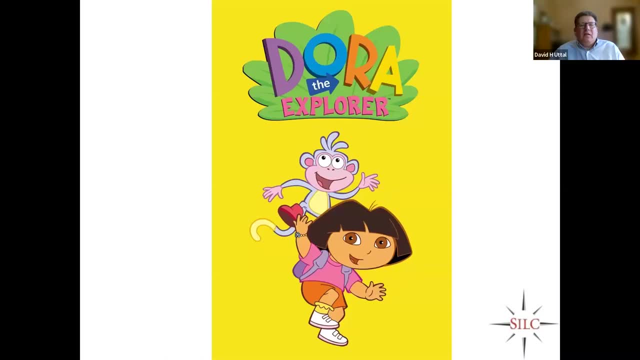 about learning about relations. So I said that sometimes, unfortunately, we emphasize object properties. It may not be the best. Stephen Freikinari and I have explored this a little bit. So if you have had kids, if you're around my age, 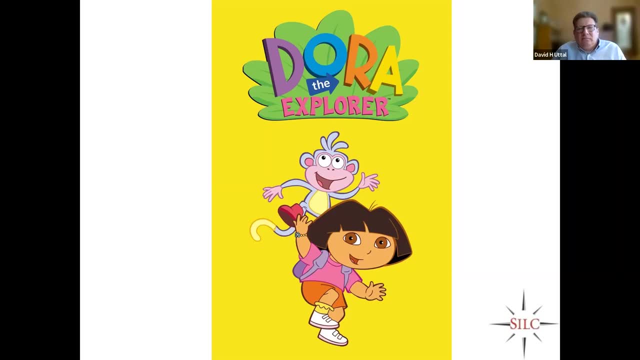 and have had kids. approximately 20 years ago, you could not avoid Dora, Dora the Explorer. Dora the Explorer is very popular And one of her several things that she does is use a map And the map comes out and sings: I'm the map, I'm the map. 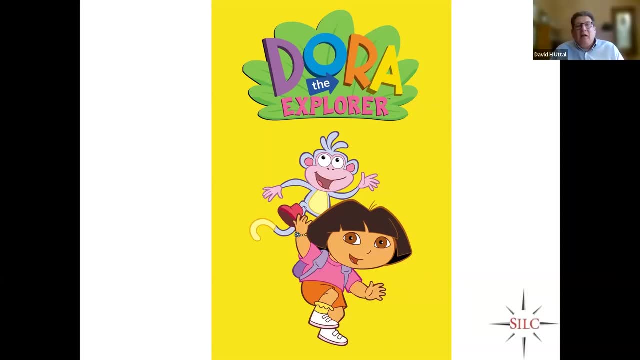 And then she says: OK, let's look at the map to see where we will be going. Well, I love maps because they communicate relational information, But the way they teach it in Dora the Explorer is exactly the opposite. So the map comes out and he shows you. 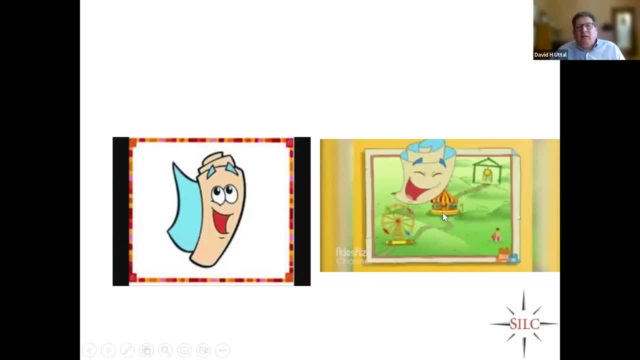 this path that says first we will see the Ferris wheel And then we'll see the carousel, et cetera, et cetera. I guess it's a little bit relational, but it's nothing like what we would typically use a map for. 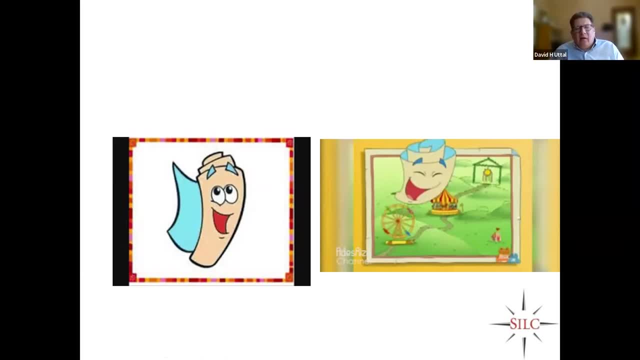 So if you said: how do I get from the carousel to whatever the endpoint is, the map is superfluous. You could easily describe that in words. It's cool that you could do it visually, spatially, But you're not taking advantage of the unique characteristic. 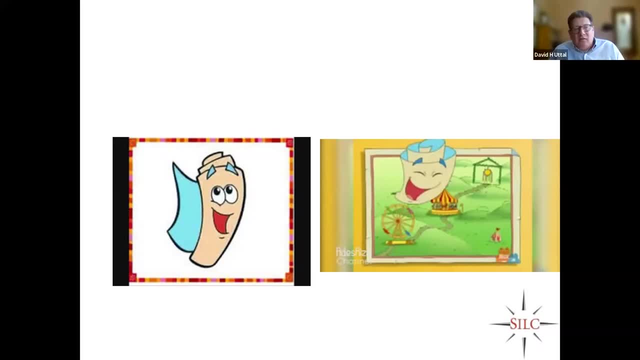 Yeah, You're not donating relational thinking because you don't need it to solve this task. When we use maps for things like where is one city in relation to another and there's multiple cities, then we're really talking about relational thinking. 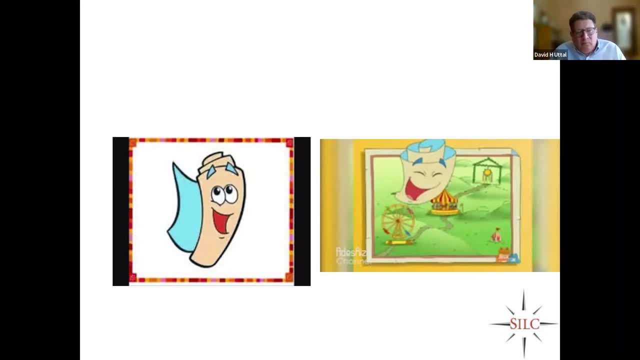 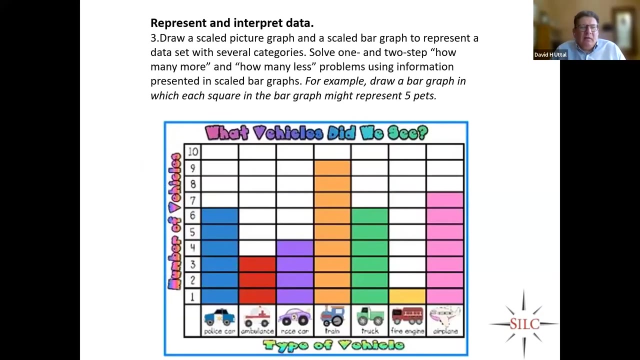 Then we really need a map, And then about half my life has been devoted to studying how using maps in that way facilitates spatial and relational thinking. OK, Another example. Another example is graphs and charts, One of the things that we do, and, to be fair, 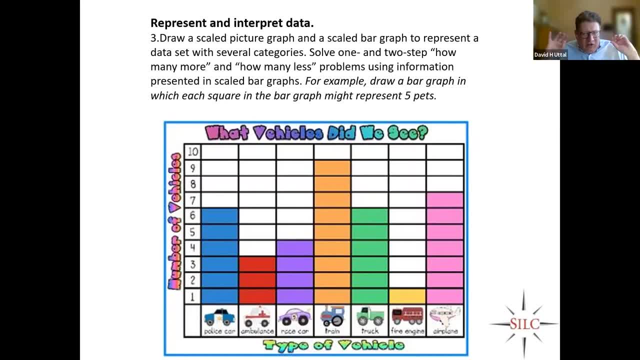 you can't concreteness fading and everything. you can't just jump into the relational structure without some instruction. So I'm not. I want to make sure that you go beyond this. You can start here, but you probably shouldn't end here. 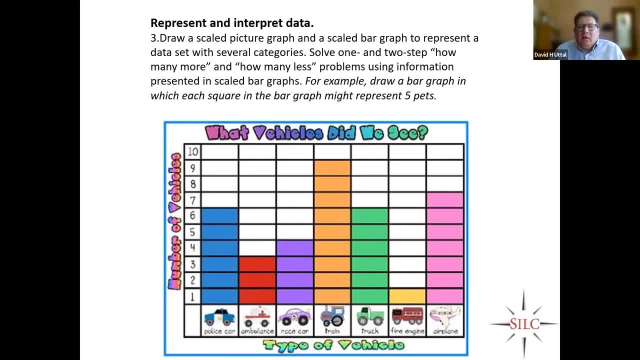 And so you're asking the kids to make graphs And this is the number of vehicles That we're doing And it's emphasizing. OK, it's mapping vehicles on two units And that's good, But what we would really use this for is 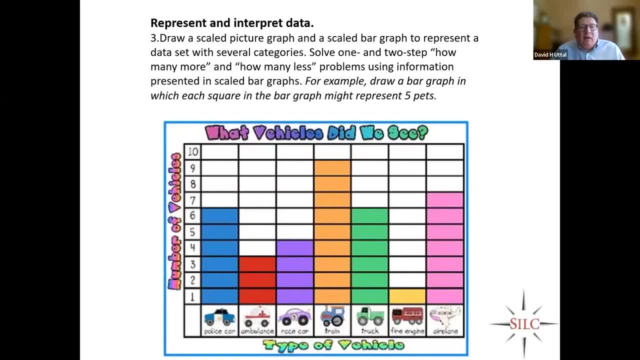 if we wanted to reason about a question such as the following: How many more race cars were there than there were fire engines, or something like that- Then the length of the bars is really, really important, And that's what we kind of use. 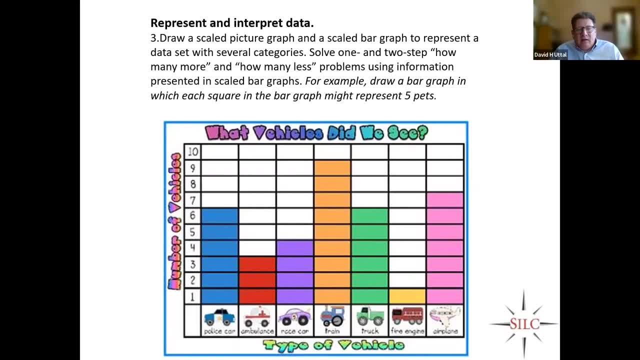 Like when we use graphs to understand interactions. we are comparing two patterns And I tell my students not to include these blocks and everything, Because what you want to see is relations between lines. Also, think about how you should arrange ascending to descending or descending to ascending. 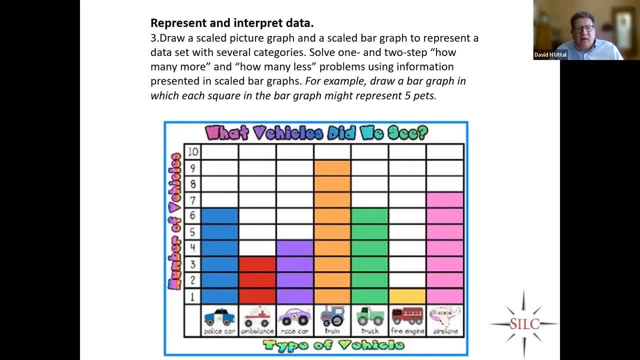 This doesn't do either one of those. So, yes, you're teaching the child how to map concrete things onto space, And that might be a very necessary first step, But the relational power of the graph is not well illustrated in this example. 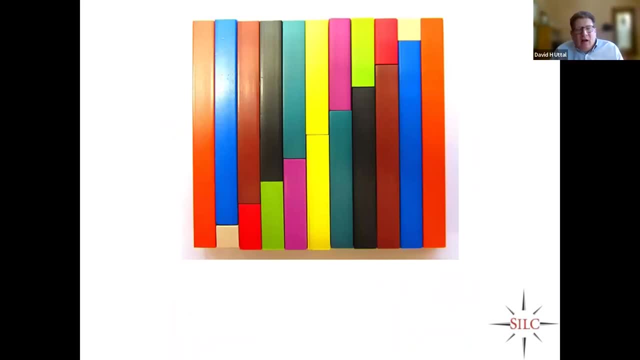 And I've written about this before- in the use of manipulatives, concrete blocks, to help kids learn mathematics. This is one of my favorite sets: the Cuisenaire rods. They can be purely relational Because you're learning about mapping different lengths. 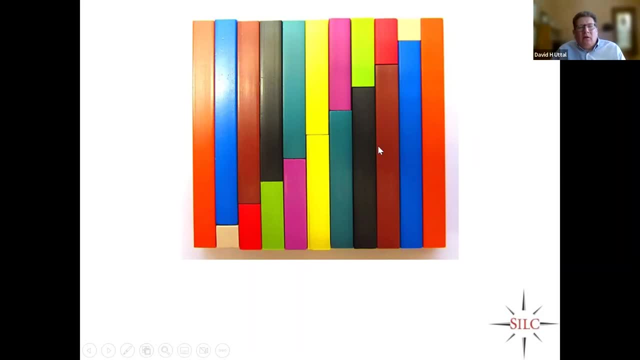 visual lengths to a different size And seeing how you can compose it, Then you can count. Say, for example, it takes two yellows to equal one red, or something like this In sort of an instruction book for using these Cuisenaire rods. 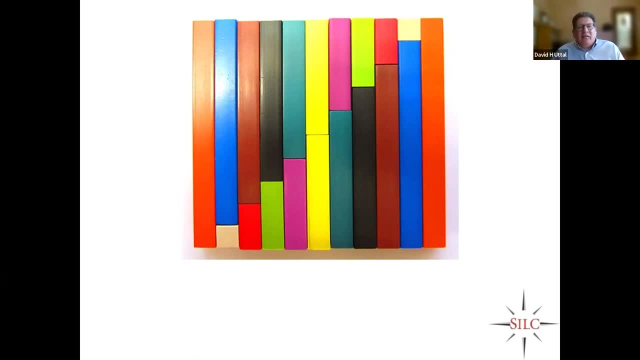 that I have. they say explicitly: do not assign numbers to the bars too early. But it's very common to say red is one, Gray, whatever color that is. Tan is one, Red is two, Green is three. And that is taking away from children thinking about seeing. 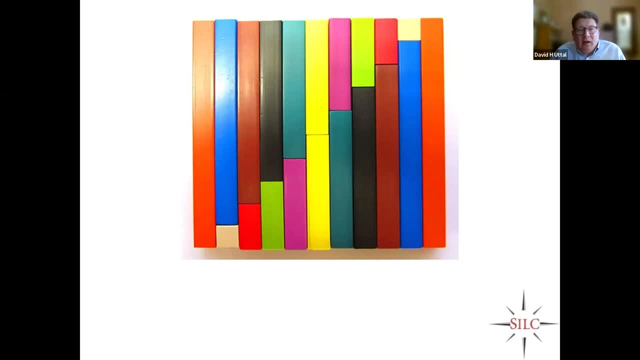 relations, seeing some initial insights into multiplication, seeing the relationship between length and then ultimately number in this multiplicative way. So when we always start with object information, we may need to start there, But we have to be careful not to end there. 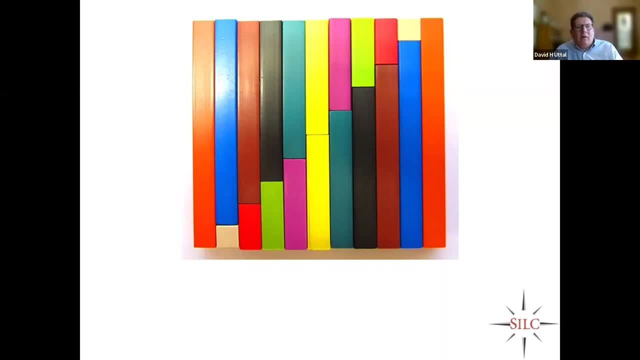 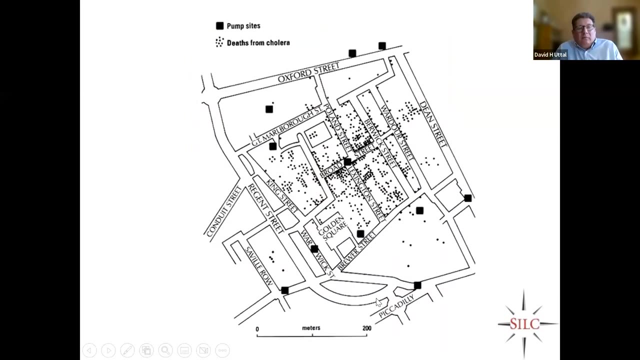 when we're using these concrete tools, Because all of these have this power to donate relational thinking. But the question is: do we take advantage of that? Now, as I said, maps- really, We are really great at this And I'm sure you've all seen John Snow's map of cholera cases. 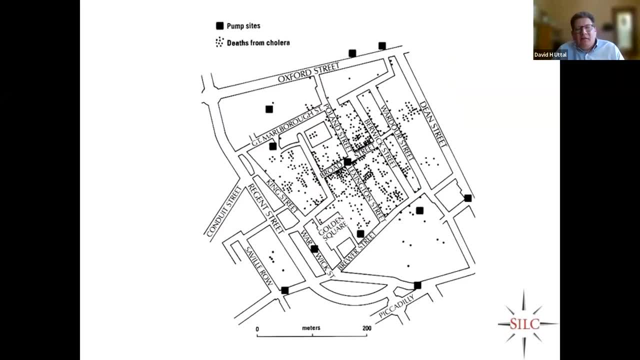 in London. This is the first geographic information system. They knew that cholera was a communicated disease but they didn't know the vector, water versus air. It's interesting we saw when COVID people actually were having not about water but air versus droplets. 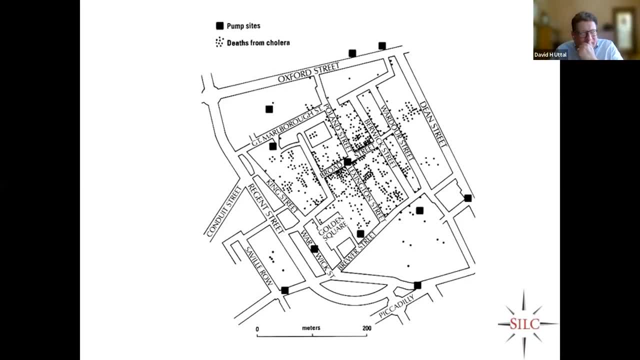 with your hands versus in the air And it took like apparently it took six or seven months to fully convince people it was airborne And apparently we want to resist the notion. that seems too magical or something They actually like to see something concrete. 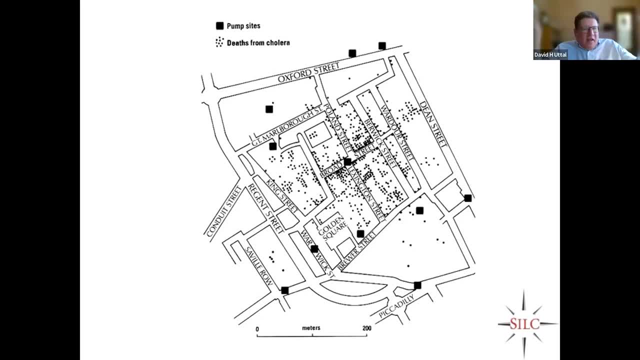 if it's an air seems unscientific or something like that. There's an interesting philosophy of science there, But anyway, eventually Snow mapped out the cases and the pumps And then the relation springs out. Then we have some alignable differences. 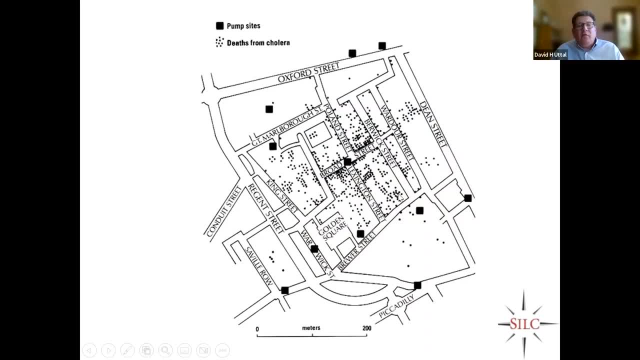 Cases where we have pumps but almost no cholera cases. And then the Broad Street pump was the central problem And everything spread out from that. In some cases people would get their water from Broad Street and then walk away. Allegedly it was the best water for making beer. 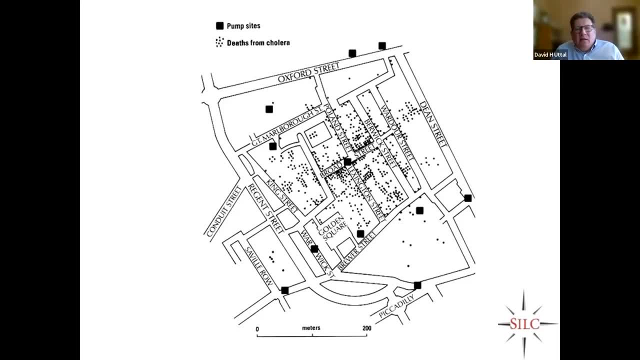 So that accounts for some of the diffusion, But the cholera cases were being spread through the Broad Street pump And the wonderful evidence that we're going to get is that the only possible elegant solution was simply to remove the handle on that pump. And the point I'm trying to make is: 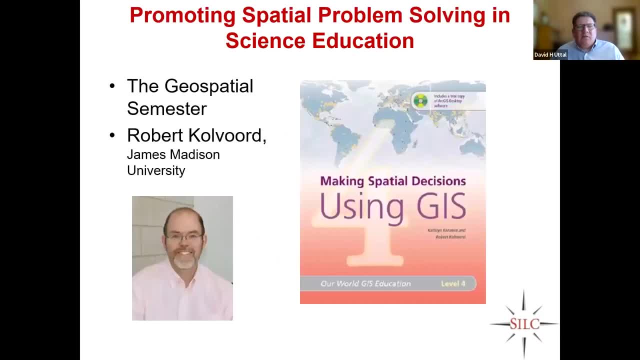 it's. the space is giving you that relational information, the spatial representation. As time is running out, I'm going to talk very briefly about some of my efforts to help students capture something of what Jon Snow captured, to promote relational thinking by using what are called geographical information. 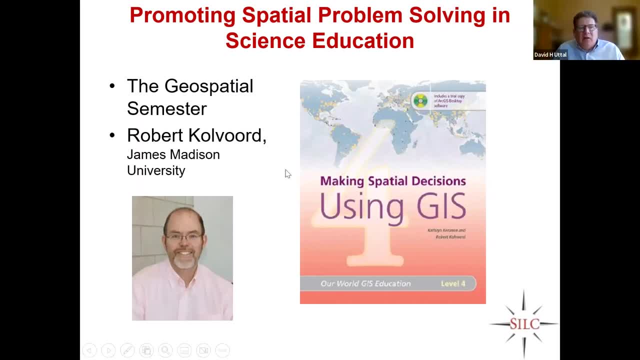 systems, And this is work I'm doing with Bob Colbert, Steven McGee and others in the Chicago Public Schools. We're doing this in what's called career and technical education, which some of you may have known before as vocational education, where the goal is more career oriented. 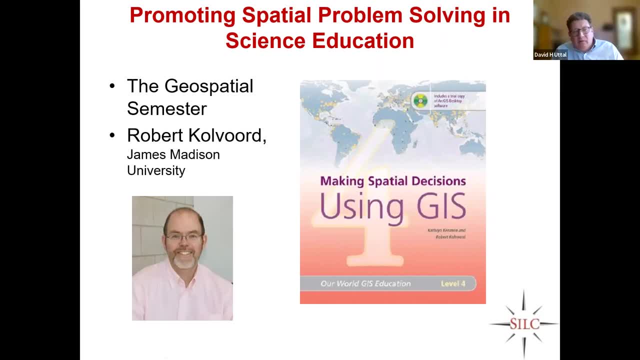 Some do go on to college, Some don't. Some go to trade schools. We're trying GIS- geographical information system- is one of the. I'm not there is one of the, but it's one of the top five growing careers. 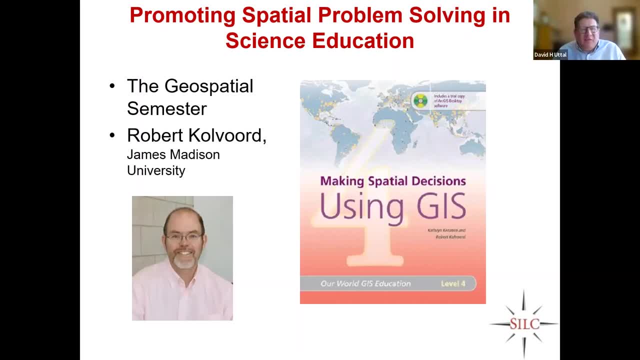 I think, after like 25 years of saying how important it was, I think it may now be taking off And it's really exciting to see, And the argument is that it promotes children's thinking about patterns and relations, which is what I say science and engineering are to some extent. 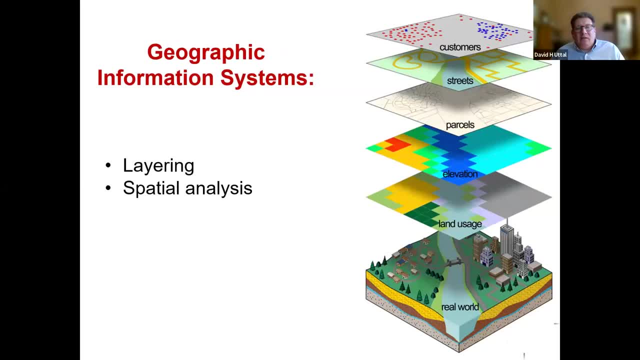 about So in a geographical information system, it's a computer-based system. It's a computer-based system. It's a system for representing spatial information, And when you pick up a paper map you're kind of stuck with what you get. 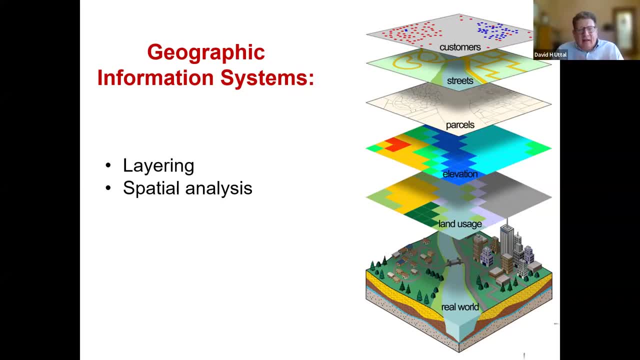 Whatever the cartographer decided to represent and how they decided to do. that is what you have, In contrast with the GIS: you choose how it should be represented and, importantly, what should be represented, And you can stack these layers and take them on and turn them. 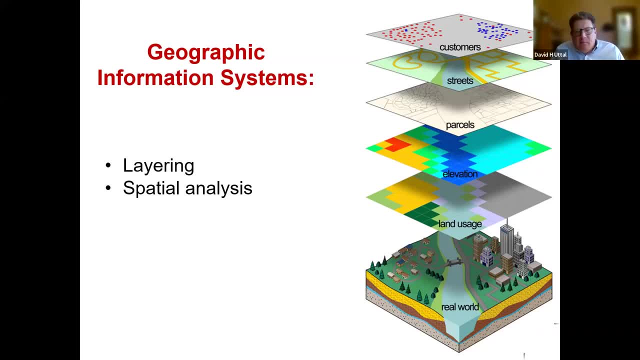 off as you're making a decision. So where should we put a new park, or a new park Or a new business, or whatever You might want to consider different kinds of information? Where is the land available? would be one of the first questions to ask. 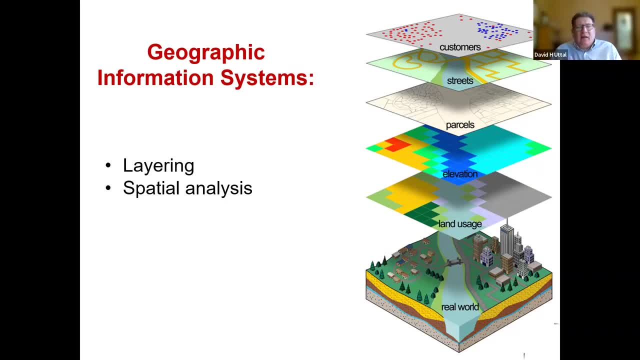 Is it accessible by streets? Who lives there? Things like that. Those are all different data sets that you can project onto the representation. You can turn them on, You can turn them off. Google Maps is a very simple GIS, but in less simple form. 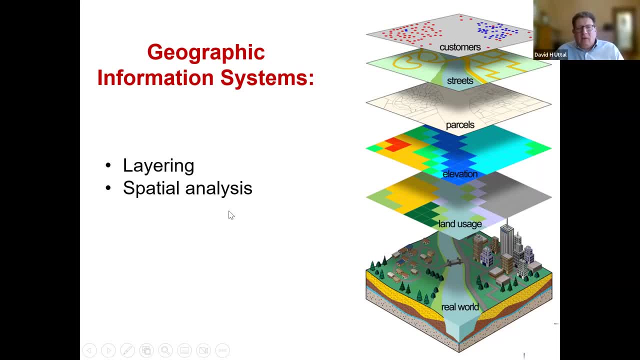 it's not. It facilitates greatly complex problem solving, like things related to climate change. Those are going to involve multiple patterns, multiple relations. It's not like people should drive their car less. Yes, that's true, That would help tremendously. 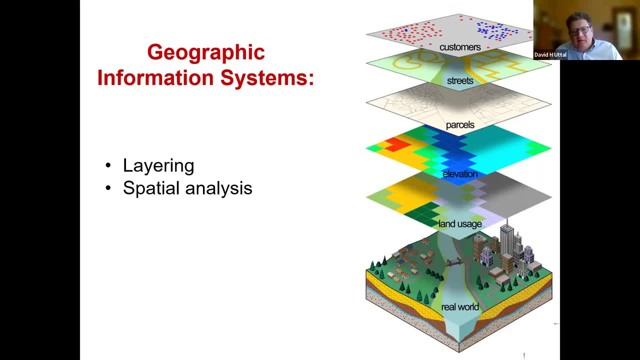 But that alone is not going to be the solution. We're going to need to consider where and how and when and why And multiple variants like that. we want to take advantage of a new kind of universal donor here, And it's multiple spatial representations. 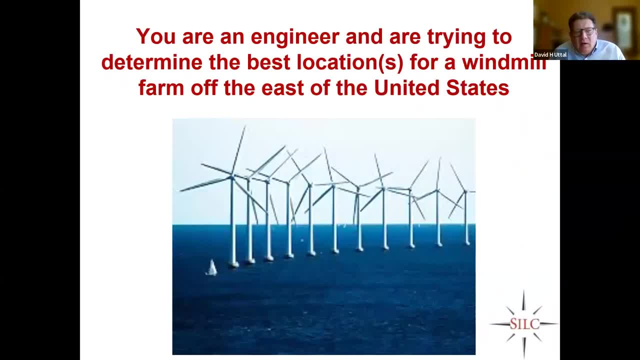 So over the course of the semester we have students think about complex real-world problems like the placement of wind farms. Now it's really a very interesting engineering challenge And one of the things I'm learning about engineering is things are constantly changing. 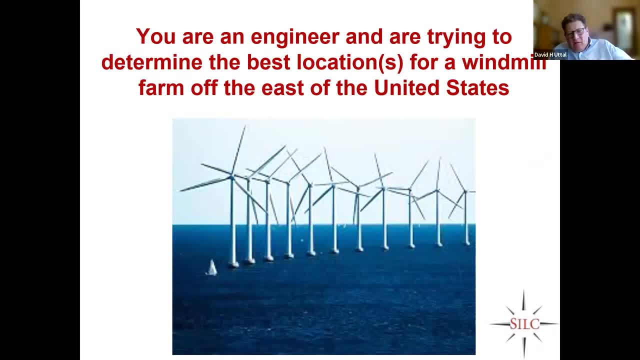 So the steel? how far down the steel can go, is a function of steel production And steel cost. it's both a trade-off of technology and economy. So how deep should we put them If we want to get them far offshore? that protects the shipping routes. 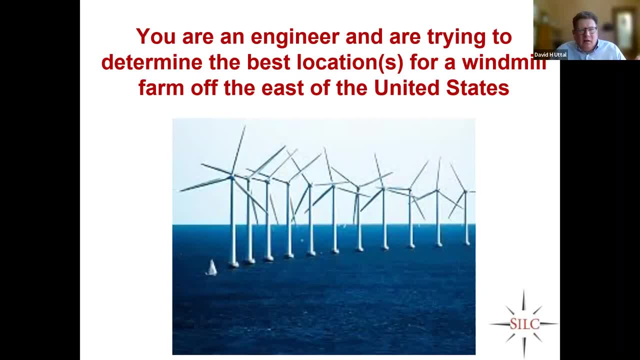 and maybe helps with the bird migration, But then on the other hand then we have a problem. They have to be more resistant to deeper levels of water. They also have to have access to the existing infrastructure somehow, So those become harder. So those are the kind of real trade-offs. 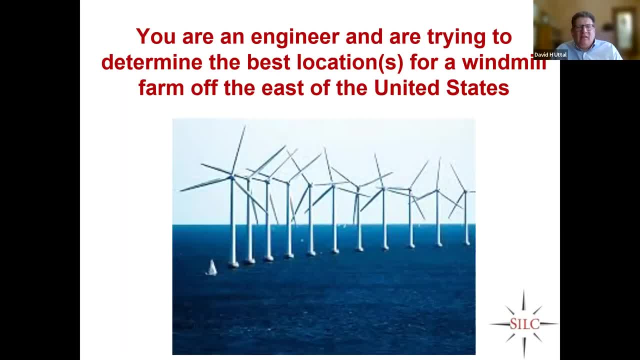 That real engineers face. Engineering is a compromised discipline. It's about what am I going to trade off to get the best I can have for this particular problem, And that's what we want them. And it's inherently spatial. It's about locations and relations. 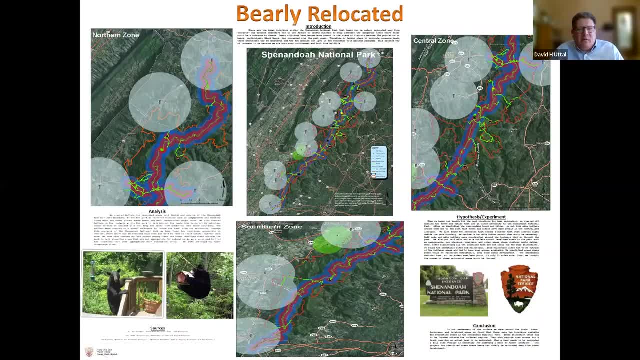 And so in this geospatial semester they solve problems like this. This is one of their solutions. a very different kind of problem, still an engineering problem. I think This is from a rural high school right adjacent to Shenandoah National Park. 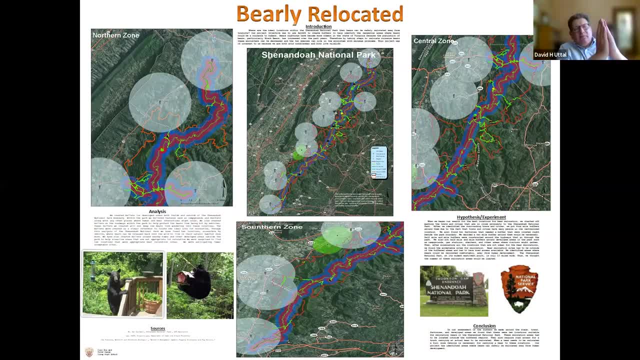 The geography of Shenandoah National Park is that it's very thin and narrow, So the distinction between what is park property and what is a village is not as great as it might be, say, in Yellowstone National Park, where you have literally hundreds of square miles of park. 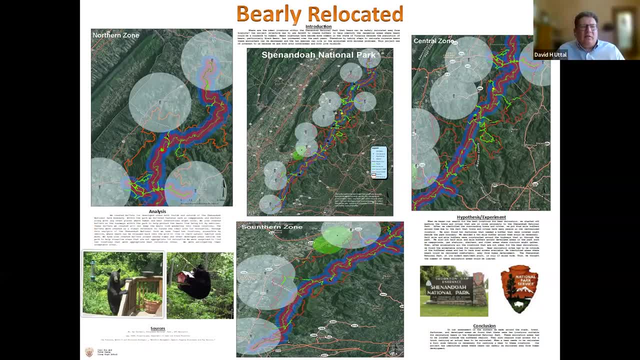 with no connection to the outside. Almost everything in Shenandoah Park is connected pretty closely to the outside, And that means the bears, who are fully protected in the park. there's no hunting allowed. There's no hunting allowed in the park. 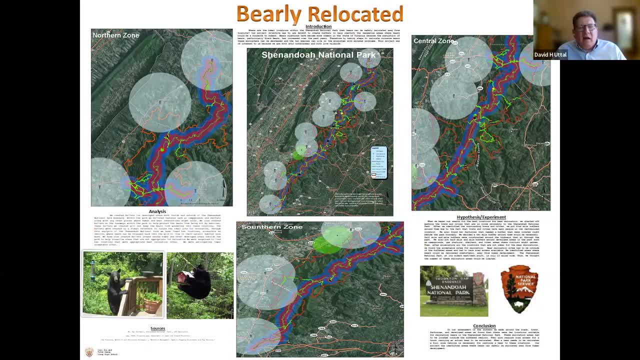 They can easily get out and into these villages And it's not good for the bear or for the people whose backyard they go into. And so the students in this particular high school. it's very close to National Park, It's very part of their stewards of the park in their mind. 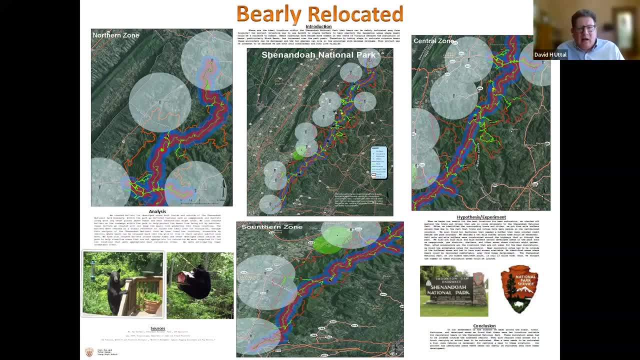 It's very part of their environment. It's part of their economic health, of their community rests upon visits to the park And things like that. So many of their parents work in the park And so one of the students said: what do we? 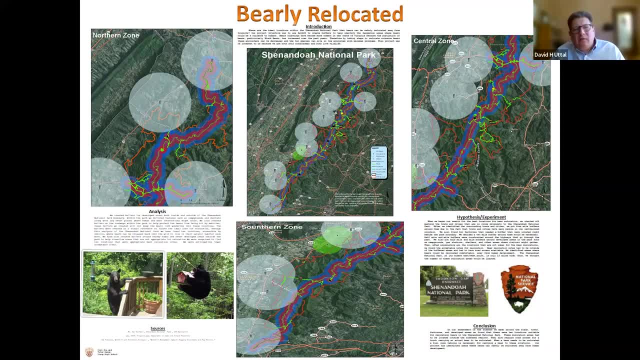 do with the bears that we catch. How can we reduce the chances of them ending up? Well, partly, it turns out there's families of bears. They're not particularly social, but they tend to stay closer to ones they're related to. 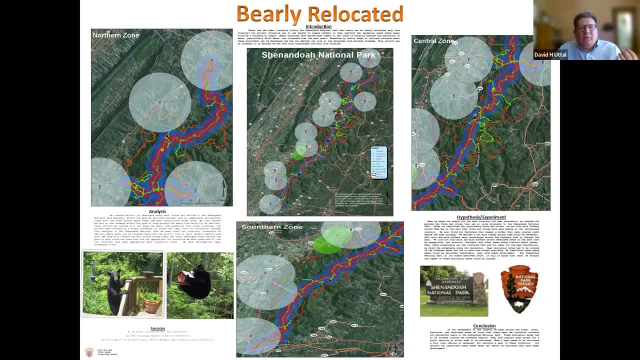 to ones that they're not. And so you have these problems of we want to put them with their family, We want to get them as far away as possible, Right From access to get back into the neighborhood as we can. You can't just put it in the back of a Toyota. 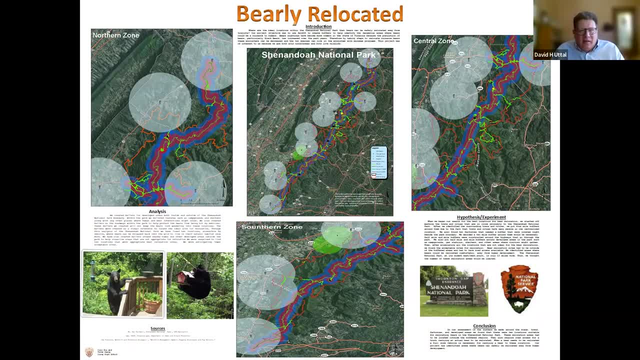 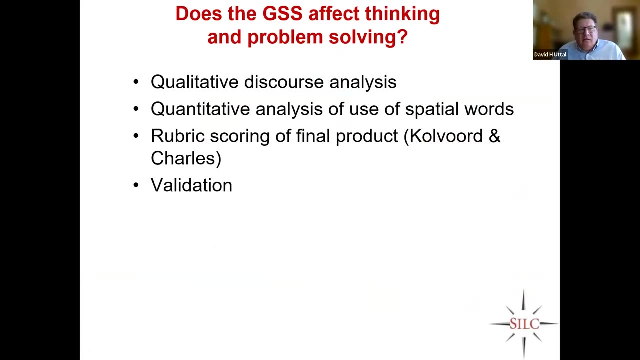 and go up the hill because it's big and unsafe. So you have to think of all these constraints And it's a real mapping task, And so this is the kind of problem that they solve. I'll skip that one. We have been assessing the effects of this course. 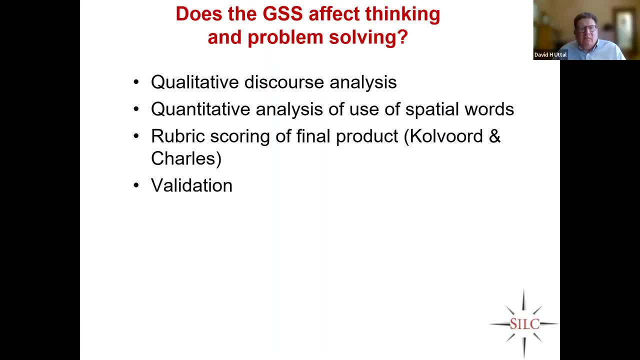 at the neural and cognitive level. Does it make a difference in health? Does it make a difference in how students think To our knowledge, and I say our? this is Adam Green, Rob Cortez, David Kramer, Bob Colbert and several others. 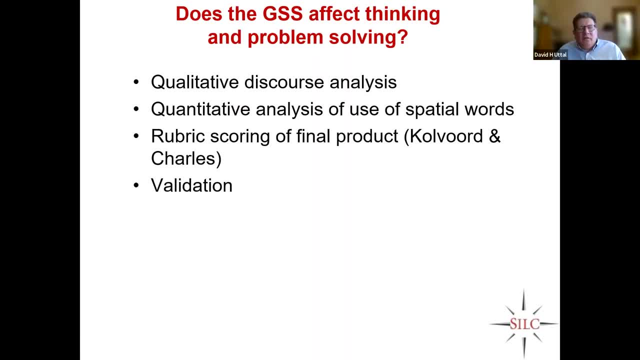 This is the first course that we know that's been assessed using neurocognitive imaging, where the effect of an entire class with any kind of control group has been assessed. Because it's hard, It just so happened that Adam Green, working at Georgetown, 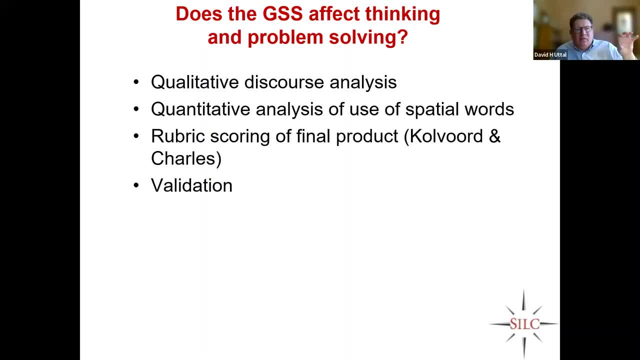 and having several kids in the surrounding suburban school districts, was perfectly positioned to recruit them and actually drive them, provide transportation for them to get from the Western suburbs of Washington DC into Washington DC and into the MRI, as well as a control group. So a control group that was taken. 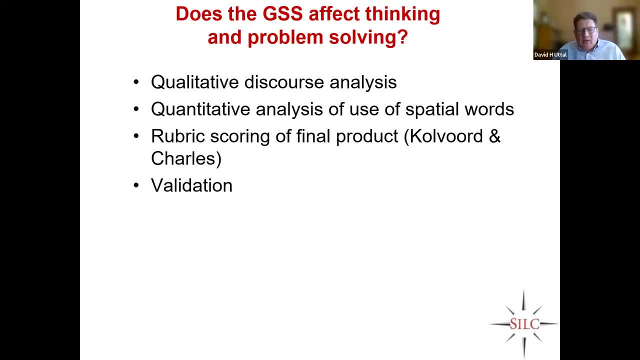 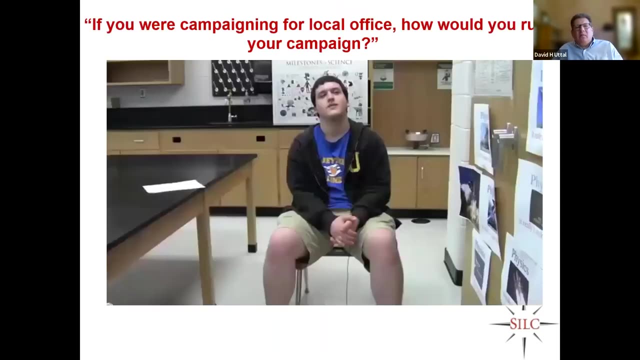 and then taking another class. So it's not a perfect control group because we can't have random assignment. We did try to use some of the modern strategies for matching propensity scores and things like that that can reduce but not eliminate possible confounds there. 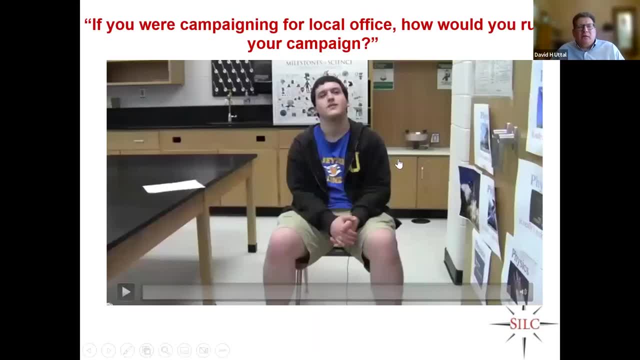 So I'm going to compare. This is one of what we call transfer questions, And we give questions to the students where they have to propose a solution. The problems are selected. we hope to be solved. They could be solved either spatially or not. 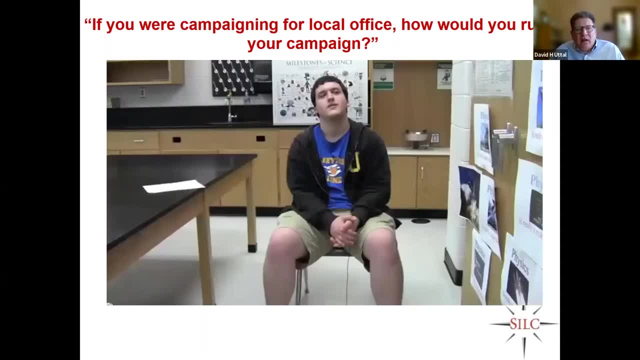 And the question is, having been in this course for almost an academic year now, do you see this problem as spatial or not? The question he was asked is: what would you do if you were campaigning for local office? How would you get the word out? 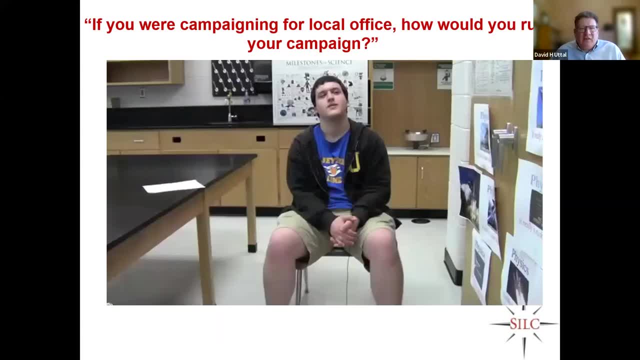 You're going to hear him mention campaigning for gay marriage. Fortunately, the Supreme Court took care of that, But unfortunately it's not. Unfortunately, you might have to do it again based on what some statements have come out. Sorry for the political thing. 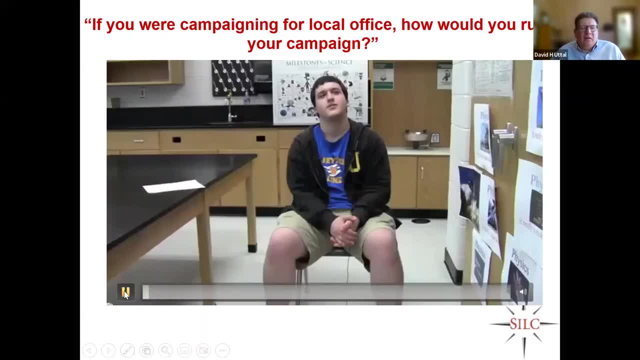 But watch his hands. He's in the map group Probably. first I would use some AGIS related to find an area that would probably maybe suit me more like. maybe like my platform, Say, like I was, maybe a small gay marriage, for example. 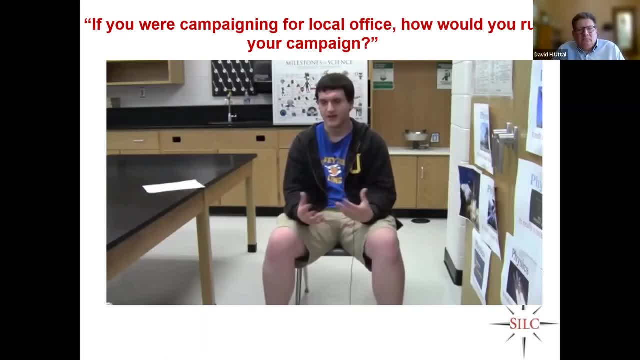 So I do like a map and I have like a poll I can find like data and like who supports it or not, and then, plotting it like on a map, I could see who supports it and then maybe campaign there, Like I'll do a lot of campaigning there. 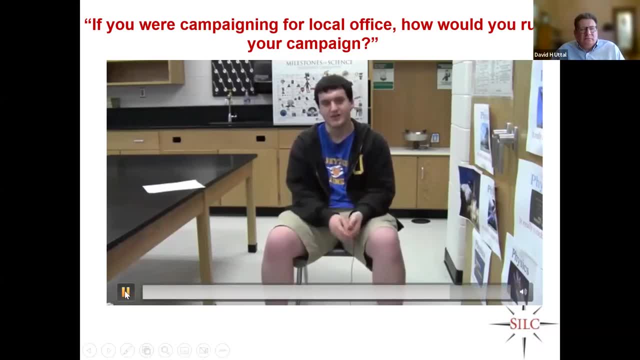 So make sure to secure those votes or something like that, So you can see to him this problem immediately is thought of spatially and through the GIS tool. How long that lasts is a really good question I don't really know the answer to. 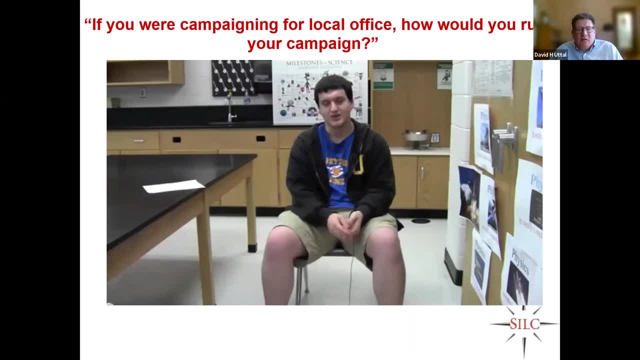 But it lasts at least portions of a school year, And so we're giving him this problem. Having worked with GIS, he now applies those techniques. Here's another student Now. yes, she's female. I'm not trying to illustrate gender differences. 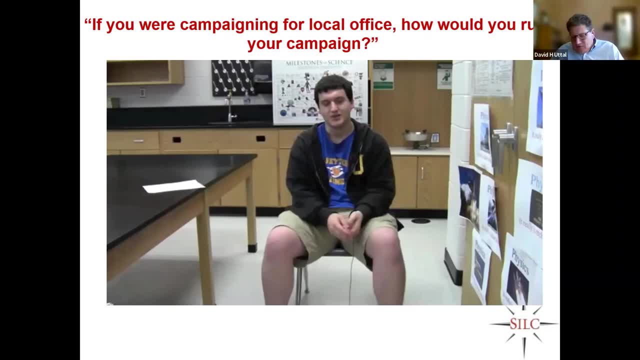 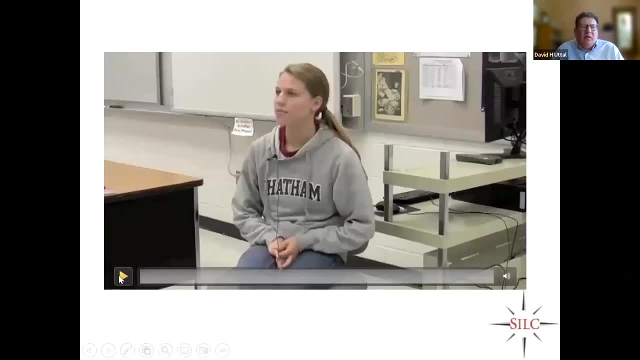 She just was a really good example. There actually are no gender differences in this, but it's just the example. So she's in the control group. The control group was either AP Physics or AP History. I could explain our selection about that or both. 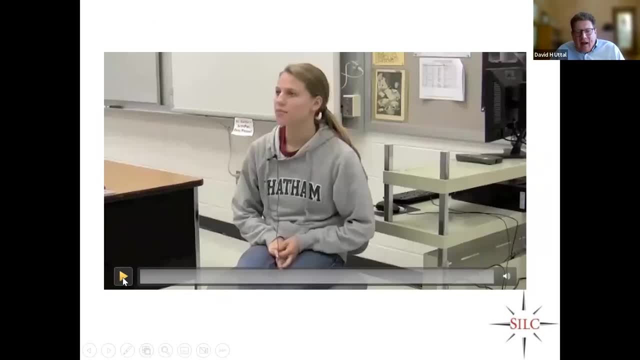 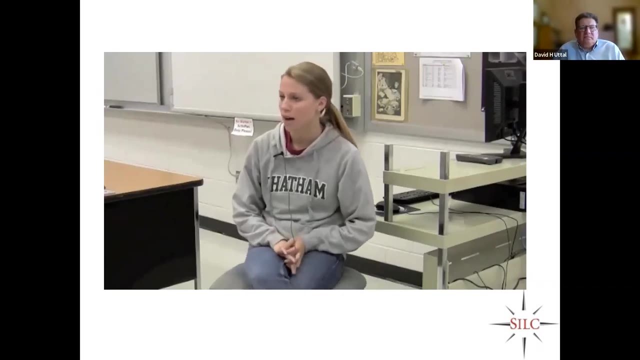 Many students take both And her answer is a perfectly good, reasonable answer. It's just not very spacial. Oh, let's look at it, Since it's local. I really want to speak to as many citizens of the town or county as possible. 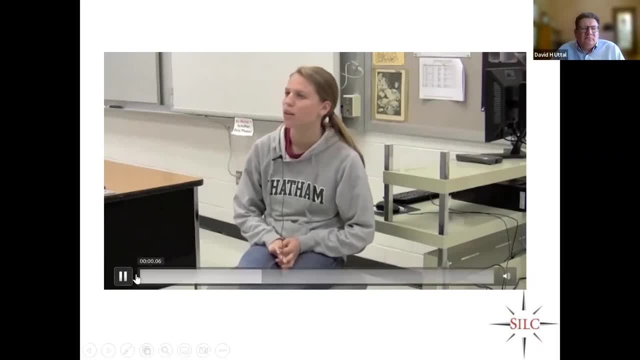 That would be very important because they would have a closer relationship with me than they would if I was running for a congressional seat or something like that. So a couple of things to note. is her answer is based on networking, which is kind of spatial. 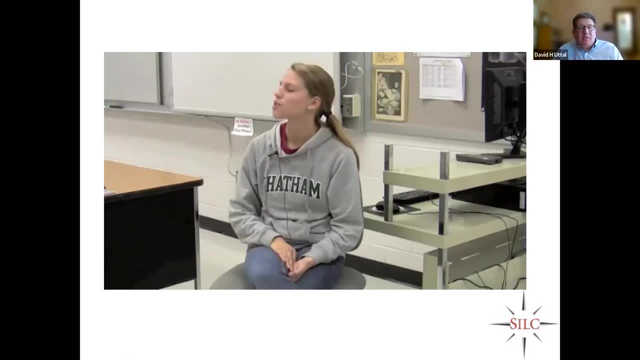 but she doesn't specify how that network would go. It's about social relationships, which is very, very spacial, And then how to sort of focus those through local businesses. The very good answer, but it's not spatial. The other thing is that her hands don't move, hardly at all. 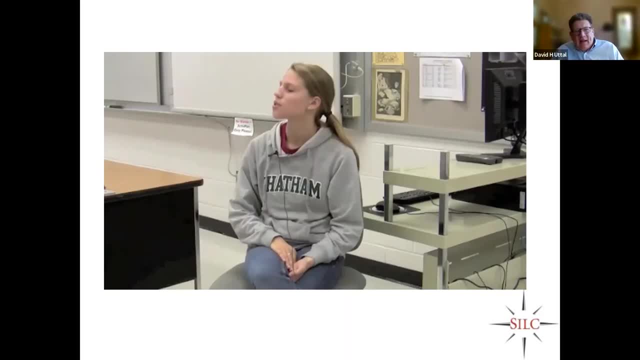 And when they do, it's what I think what's called a dietic gesture. It's kind of like just pointing or beating to keep the speech going, whereas the first person used his hands to illustrate a map. And we have more evidence than these two anecdotes. 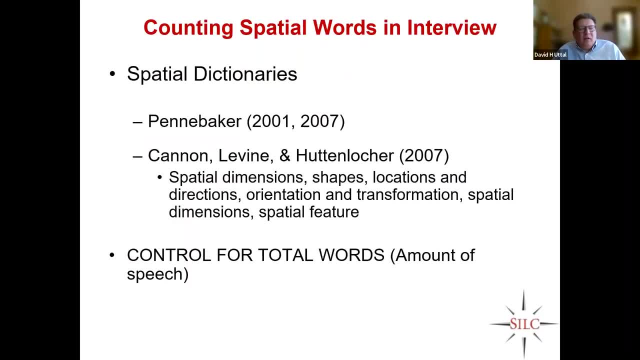 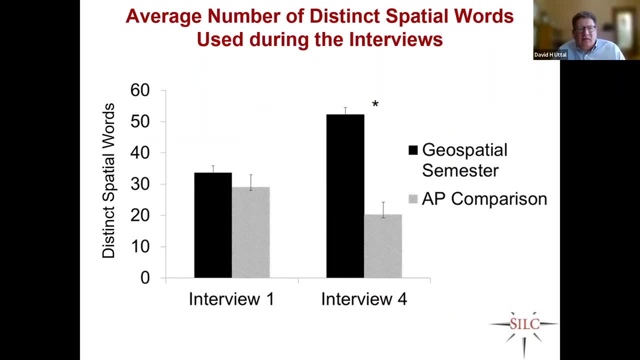 to suggest it's actually making a difference. I'm running out of time so I'm not going to go into detail, But we have four interviews across the quarter where we ask them questions like this And one simple measure based on work by James Pennebaker. 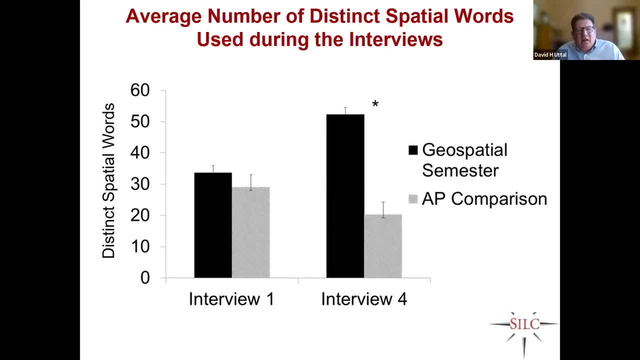 basically, what people talk about reflects how they're thinking, And we can use dictionary as a spatial word. So basically they're thinking more spatially And the control group is actually thinking a little less spatially, although not significantly so. So this big difference between the black bars- 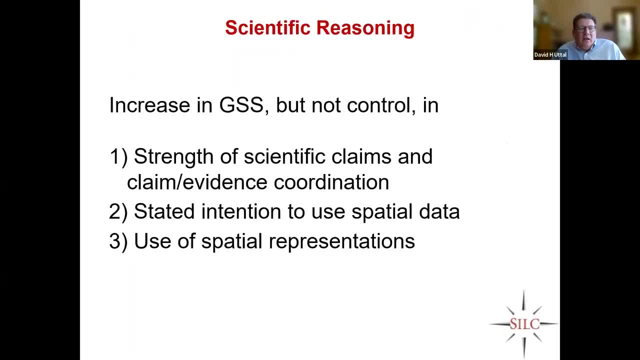 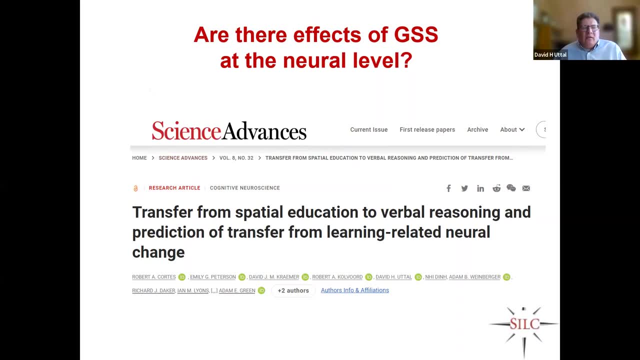 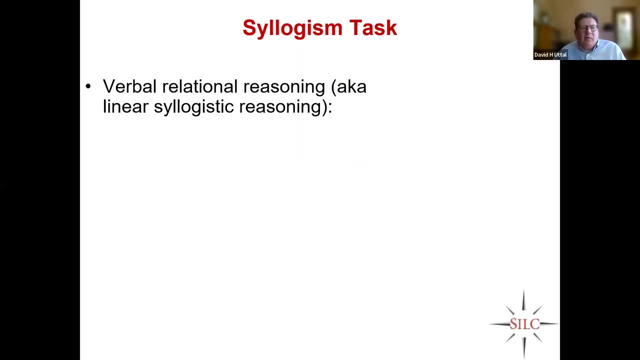 is illustrative. It's just that something changed, And recently this just came out- It's online. Science Advances is Rob Cortes' first author, where we looked at neural and cognitive or behavioral measures of spatial reasoning and used syllogisms here. 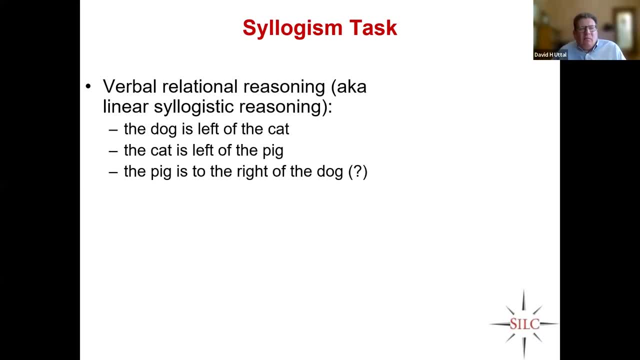 because that's even more removed from the actual specific problem. This is a spatial syllogism where basically you just say yes or no And we can measure. We can measure your reaction time. There's a huge debate about whether people solve these propositionally, spatially or both. 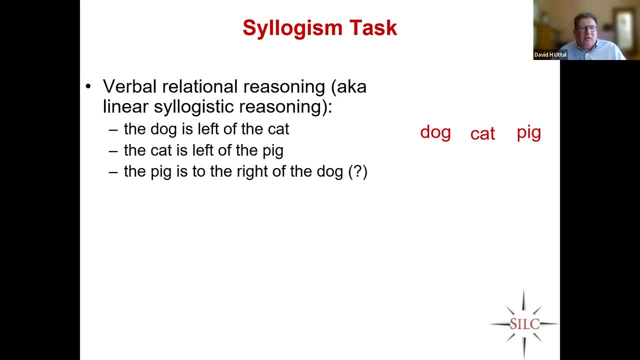 I think what we can say is: after they take the geospatial semester, they're more likely to solve them in a visual, spatial manner. The areas of the brain associated with that are more activated And areas that are more associated with verbal processing are less activated. 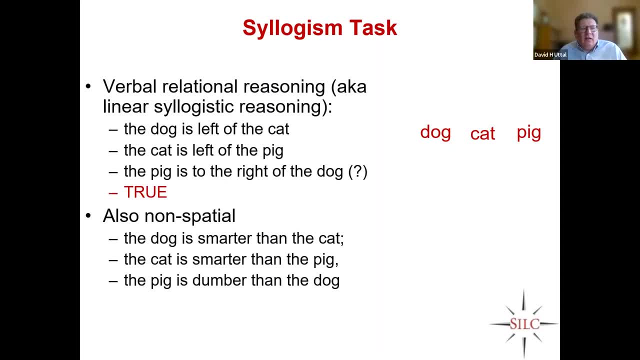 And you can read about that in the paper that's just finally out online. So they also very cleverly came up with non-spatial relationships and showed that even the non-spatial syllogisms are solved more spatially with more relevant brain activation.